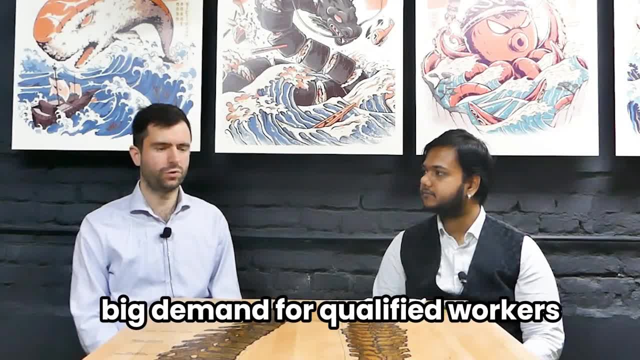 I can see currently there's like big demand for qualified workers, like both qualified and unqualified. We would be actually like giving you insights as of 2024, this like how much you can make as well from each of these jobs. Students, because they see some money and it's really good. 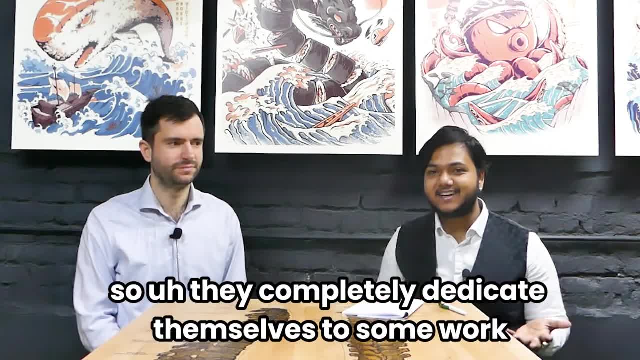 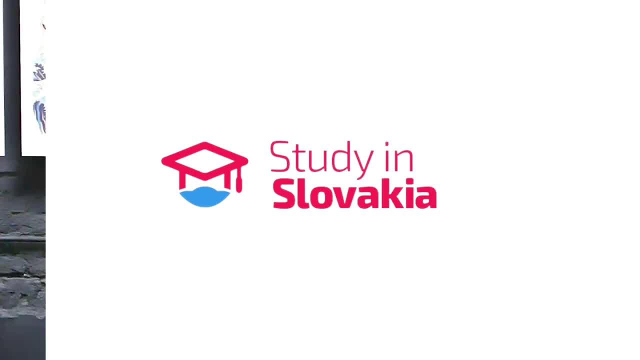 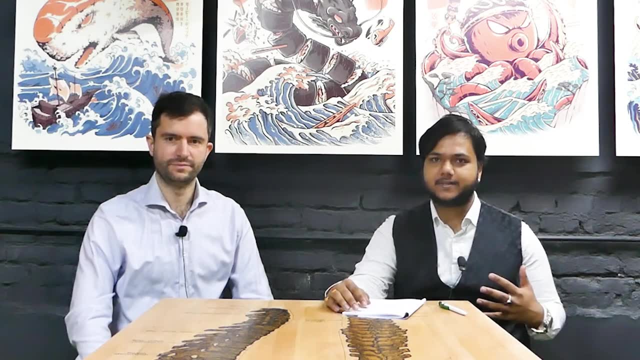 money. obviously it's in euros, so they completely dedicate themselves to some work and then ignore study. Hello and welcome to Study in Slovakia. Today we are going to cover a much awaited topic, which is about part-time jobs. This is a very common question almost in every video We have. 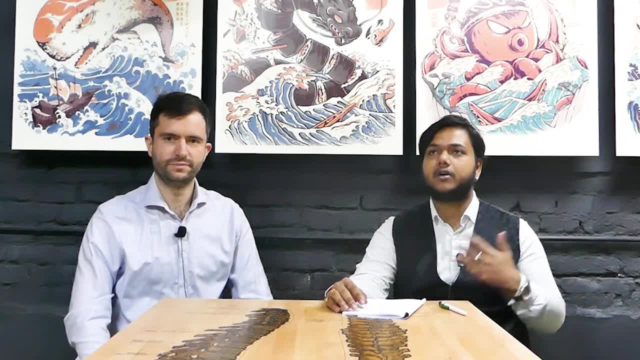 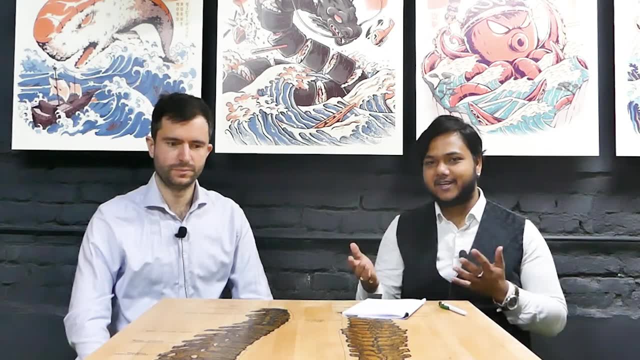 some comment, or you know someone who's planning to study in Slovakia or international student always has this question: What are the part-time jobs? What are the available scopes? How much can I make from there? Can I manage my living expenses? So today we have Mr Peter with us. Mr Peter, 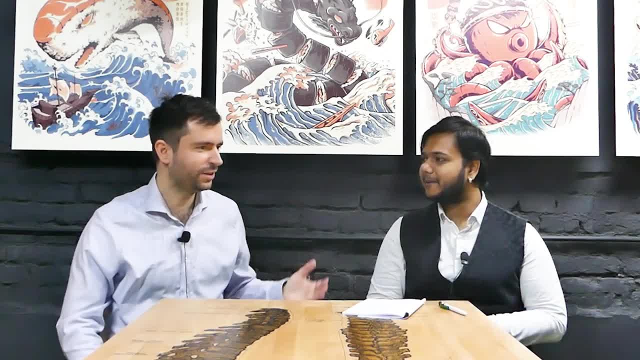 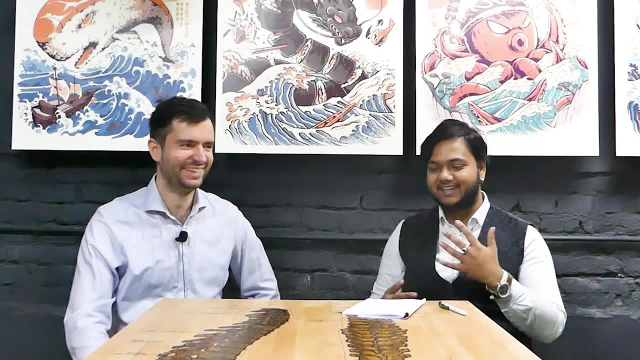 thank you so much for joining us. Thank you also, but I think you will be the person with more experience And you're the person with the connections regarding part-time jobs, because I expect like people are reaching out to you regarding part-time jobs mostly. 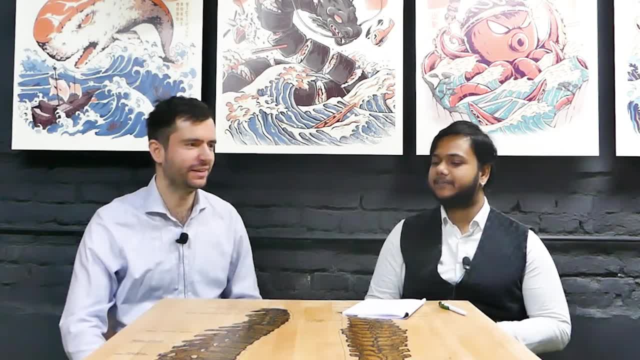 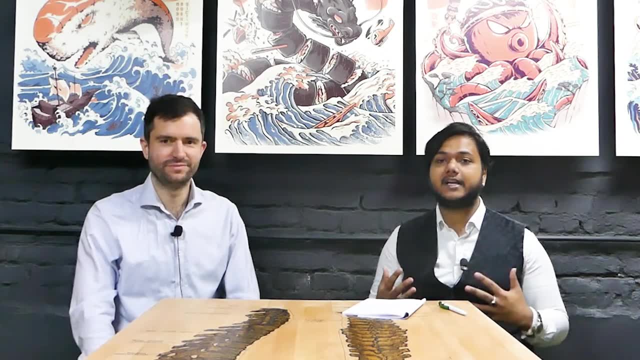 They do. I can share my experience and we can then compare. Yeah, sure, So we will be diving deep into it. What are the different options, and can you actually rely completely on part-time jobs when you're moving abroad? So this is going to be. 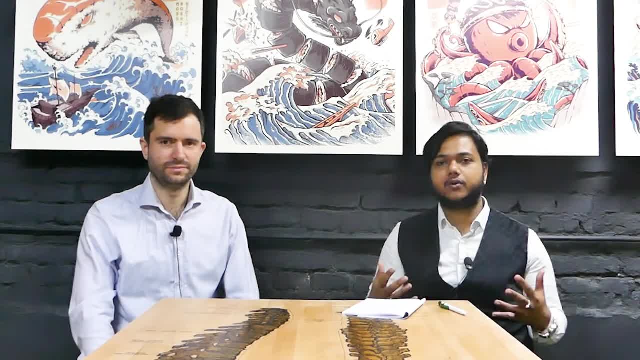 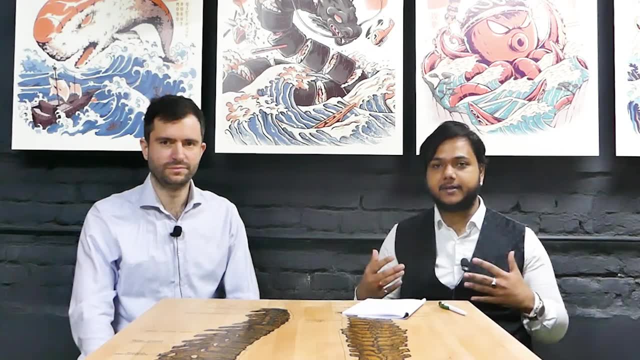 obviously focused on Slovakia, but there's also a general question about the part-time jobs. So can you make it in Europe? Can you like, for example, sustain a life in Europe just based on the part-time jobs along with your university studies? So, without further ado, let's get in. 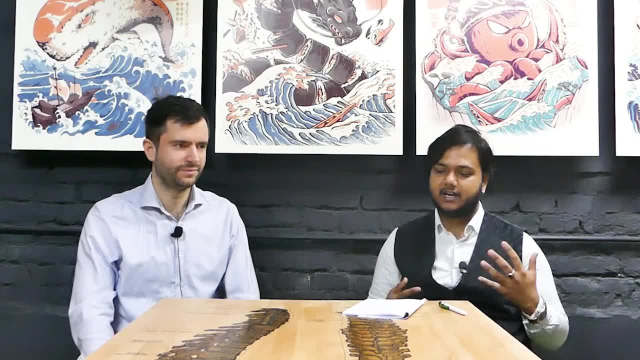 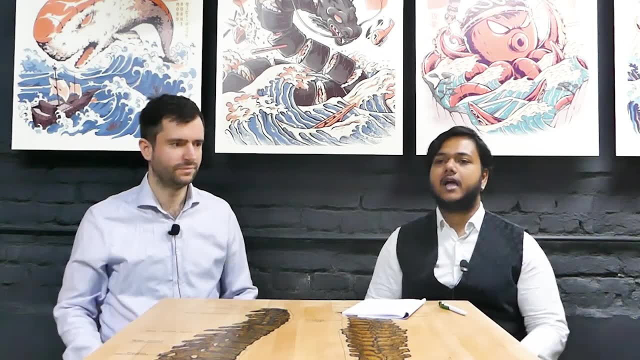 the video. So, Mr Peter, starting first things first. like what are the available jobs? I would like to classify some of those which I personally know, And I see many of my friends working there. even when we were students we were doing the same. So there is obviously 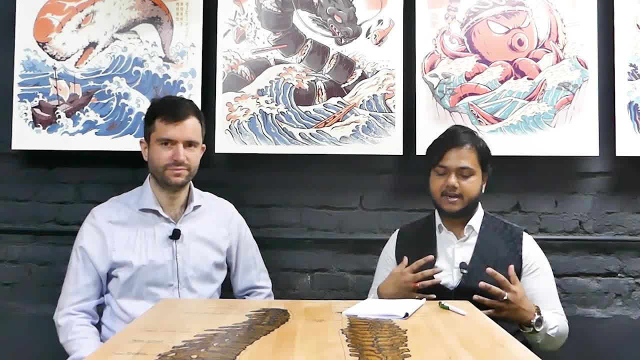 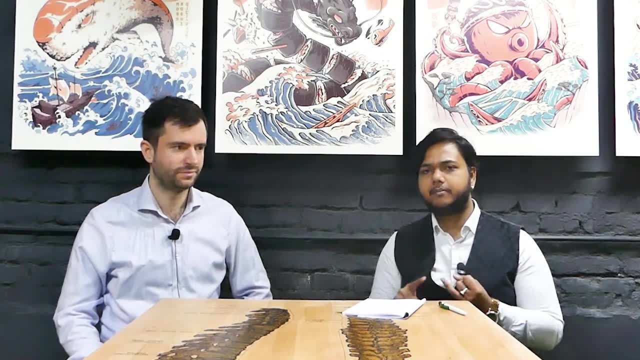 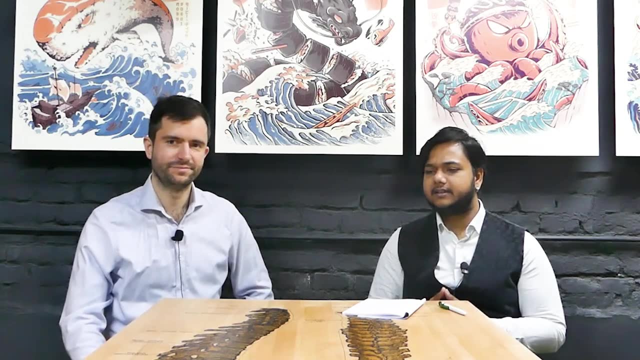 some jobs which are commonly available and, you know, easily accessible for anyone. something like deliveries which is done by foodora, foodpanda, bolt, volt, uh, then bistro and so on, yeah, and, and also taxis. regarding it, uh, so it can be like taxi driver or like delivery operator with a 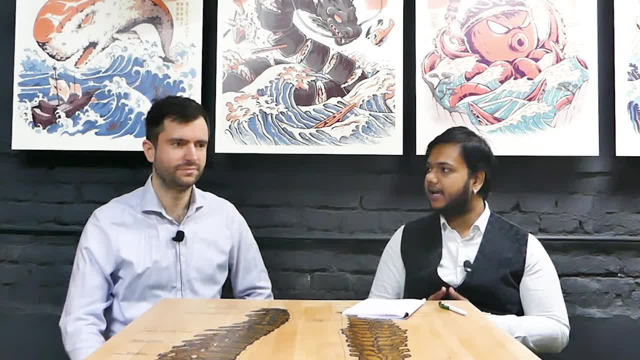 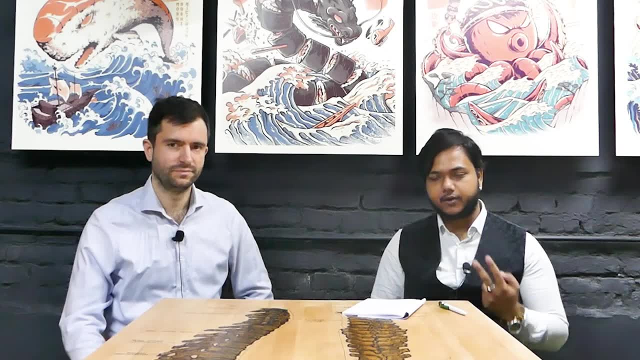 bicycle. this is generally very easy to break in, and that's uh one of my insight that i uh find. um, it's obviously like there are two options how you can join it. one is you become a sole proprietor, in which case you can maybe give us some insight. i guess we don't have to change visa. 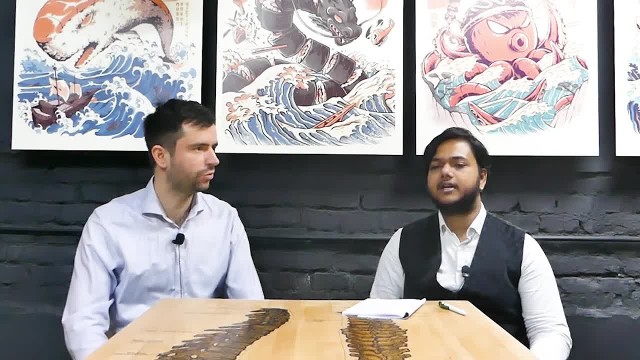 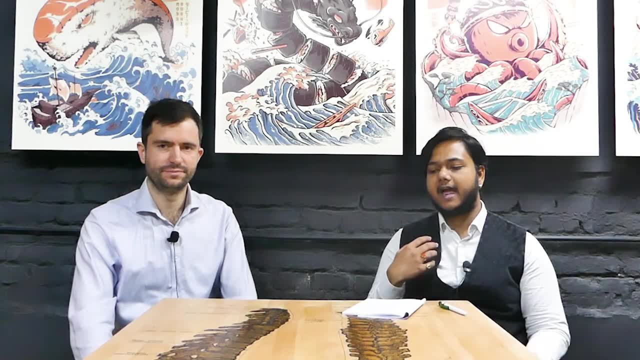 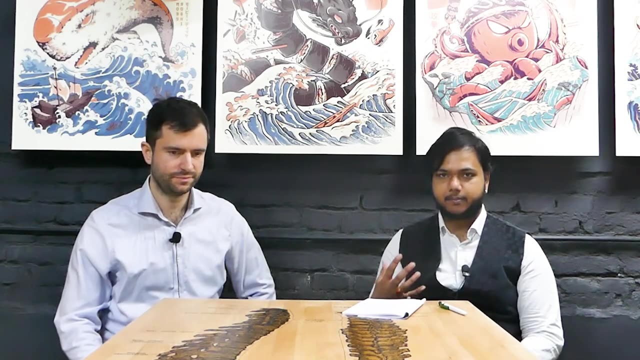 in that case, right, as a student, you can also run business. so either sole proprietorship or sl. yeah, so we can uh actually be students and uh like we can still uh, for example, run as a proprietor and uh we can do as a as proprietary. it takes about seven days or maximum. 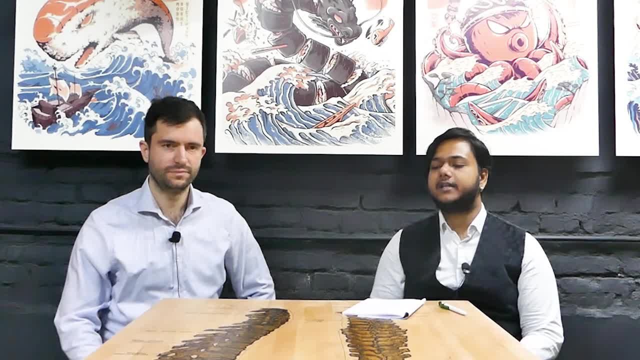 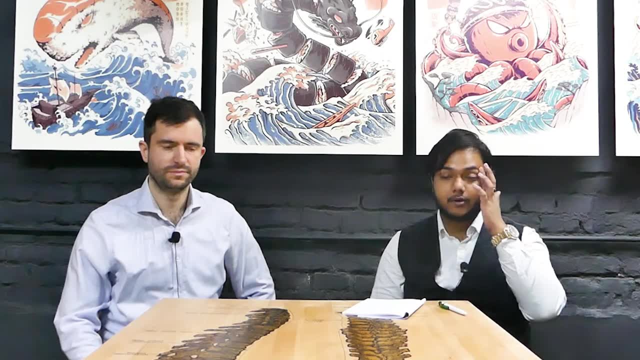 like two weeks to like set up this and you're good to go. the other option is there are some third-party providers, third-party agencies uh, that are there, online, available when you submit the form in any of these applications. uh, that will cut a certain percentage of commission. 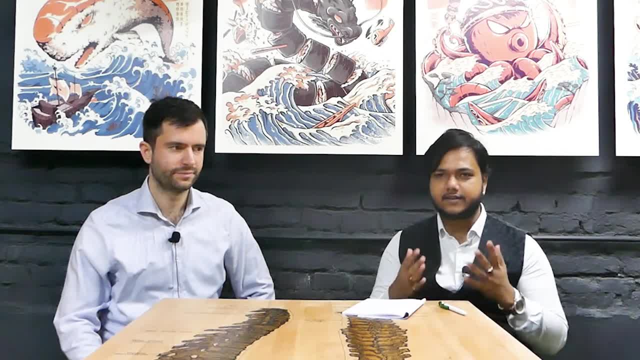 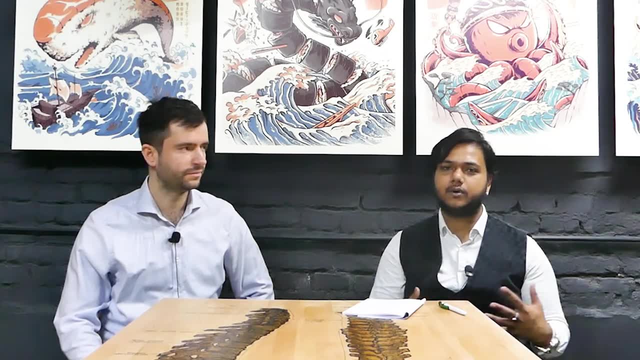 that might lie something around like 15 to 20 percent, around 17 percent. many times, uh, that is going to cut this commission and then going to pay you the rest. in that case you don't have to do a manual registration and everything for your business. the difference what happens is generally when you start your business. you might have to do. your get your accountant, have your tax filing, obviously pay for your insurance and everything comes with it. but when you're like uh, doing it under like some agency, you generally don't have to do these parts because the accountant lawyer and everything is done by. 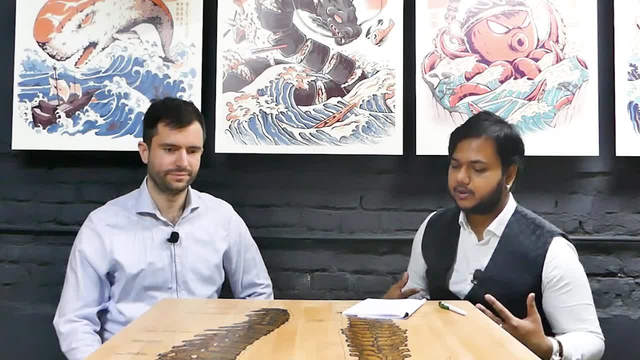 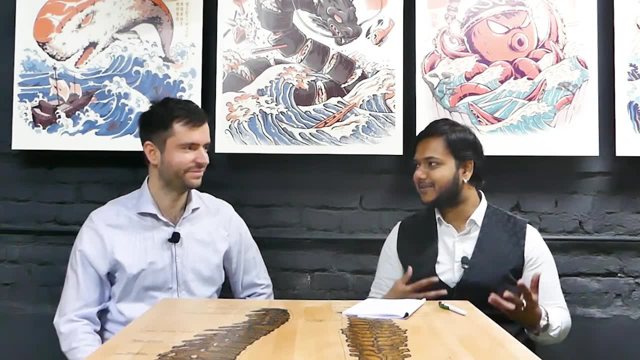 the agency itself. so it's uh generally a combination of both. the other is, uh obviously there are restaurants. now, as an indian, i can say there are many indian restaurants also, like if you're coming somewhere from asia, there might be uh many irrelevant and you might have a community there. so to reach out, 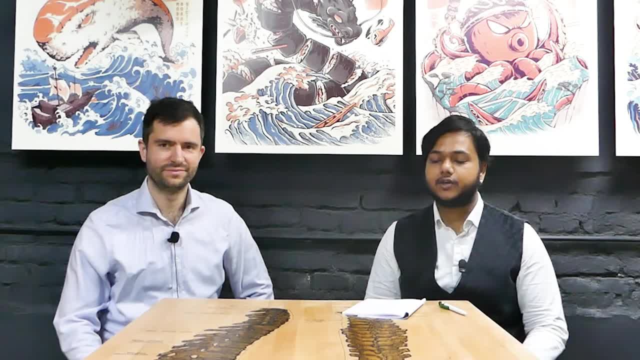 to your local restaurant or something. this might be a very good place for you to build a community and from there you you might find- actually like the majority chances are you might find- some part-time jobs from there, like that is a general trend any uh country that uh students are going. 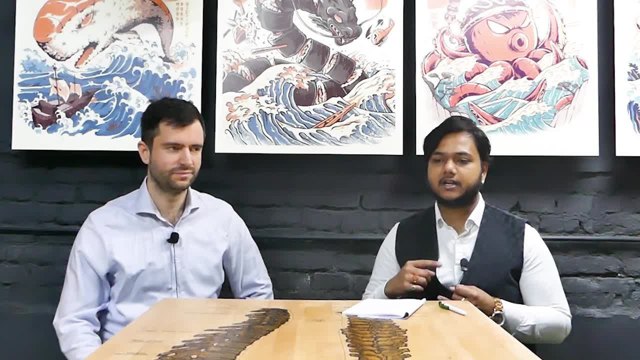 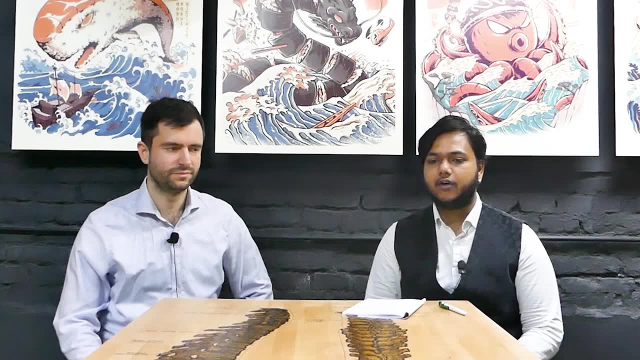 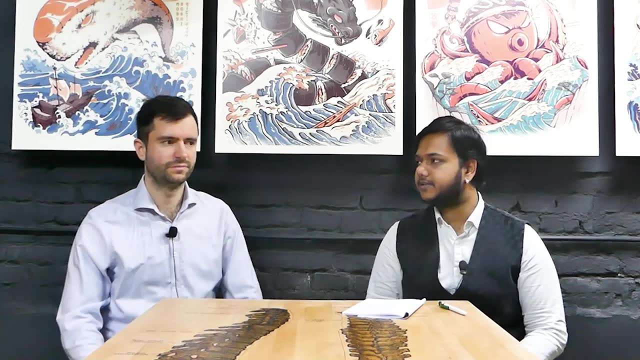 restaurants are like uh, whether like it is servers, whether it is uh, for example, kitchen helpers, it's generally like a easy job to uh have at first. uh, obviously, the like uh pay uh varies from like the delivery to this thing. well, for the delivery, one thing: what is very important is you need to 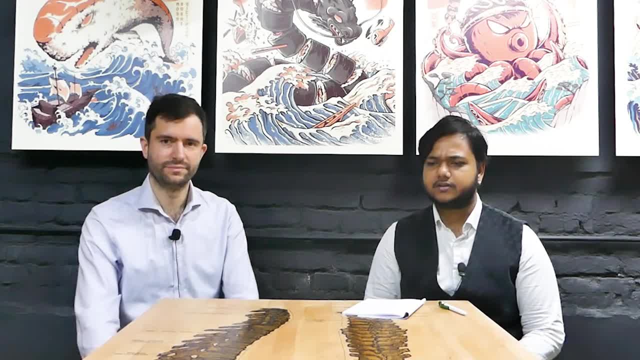 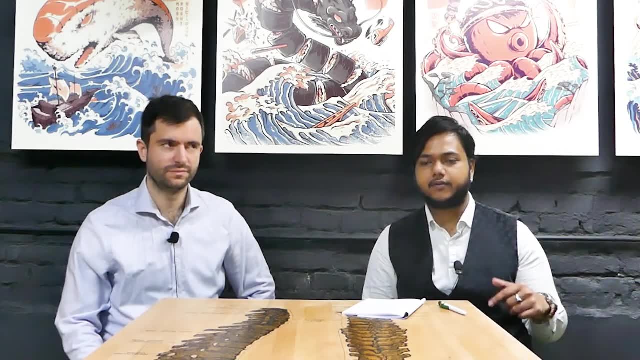 have a bike or bicycle, uh, for that, uh, it costs you like max, let's say, 50 to 100 euros to buy a second-hand bike. we will provide the link in the description for a website called puzzles, which sells these sort of second-hand bikes and everything. uh, that might be relevant for you. 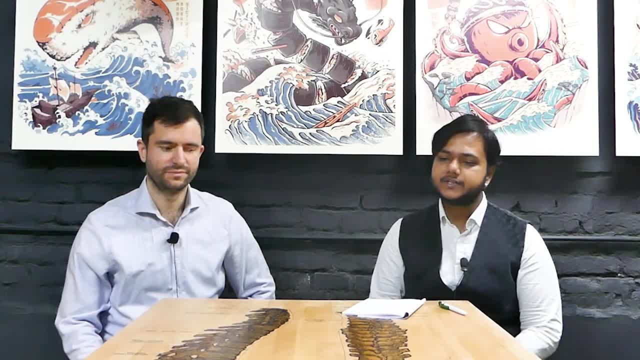 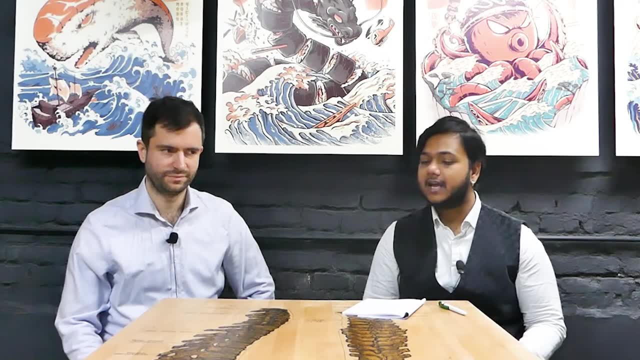 and you can quickly like purchase from there. once you're uh like good to go with this, then there is another option, if you have a little more money, is taxis or, for example, commercial vehicles, but for in that case you actually need a driving license from your native country. you need to recognize it. 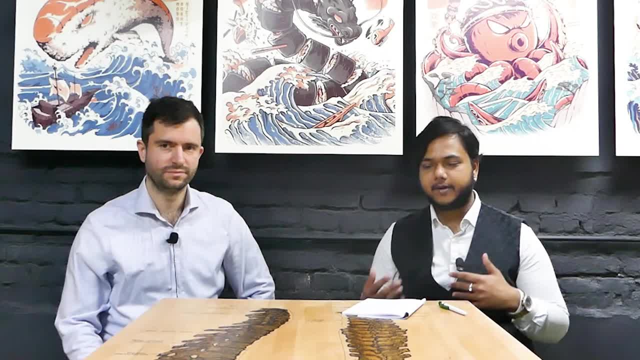 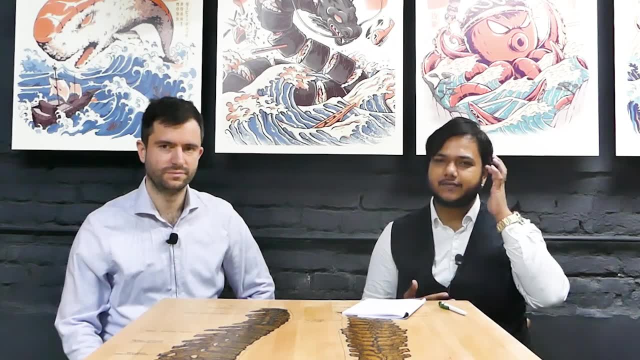 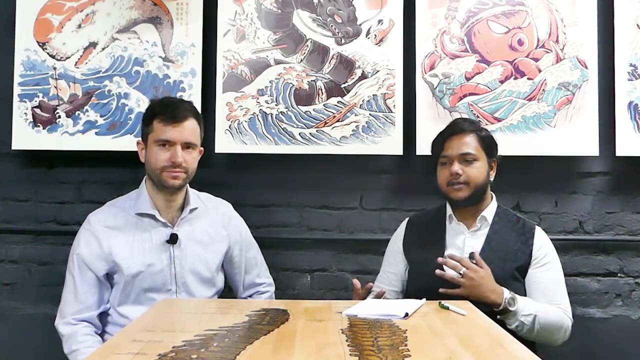 here, change it to the european license. it is a little bit of paperwork, firstly. secondly, you might need to purchase a car as well. you can rent it as well, but a general purchasing car is not very so this is one other way that you can do. now mr peter will give us some insight about uh doing. 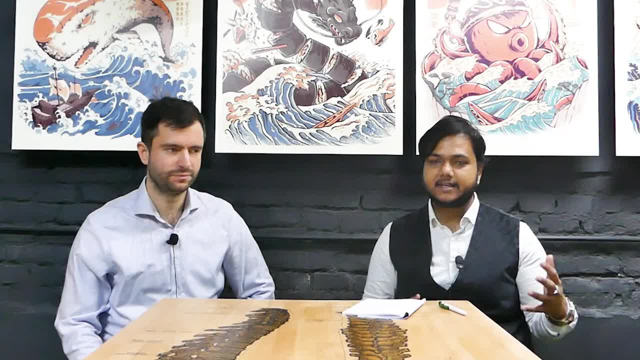 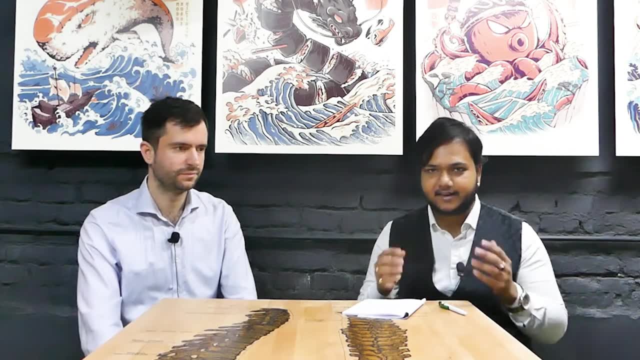 some jobs that is relevant to your industry. this is something you can do for survival. it means, like you will obviously have the money for your food, your accommodation, your uh, let's say, extra partying and everything. uh, this is generally enough for it and obviously this is something that you can. 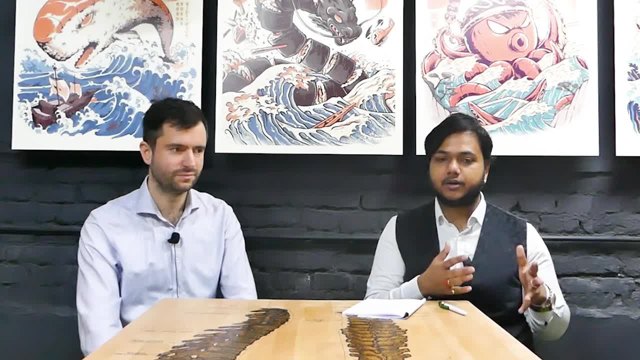 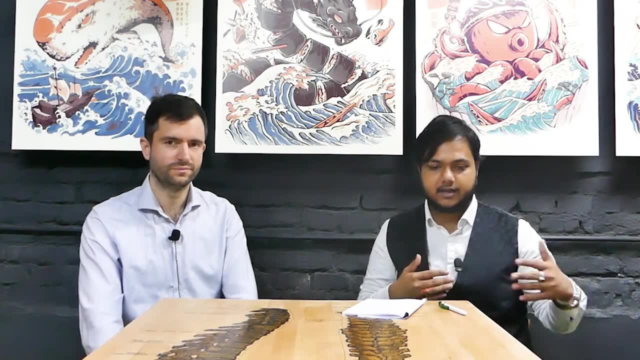 have throughout the year. but there are also jobs, which is very important for you to progress in your career, which is actually going to take you through the career path, and you can do that by- and you know, push you to the full-time jobs that you're actually, uh, studying for your, um, you know. 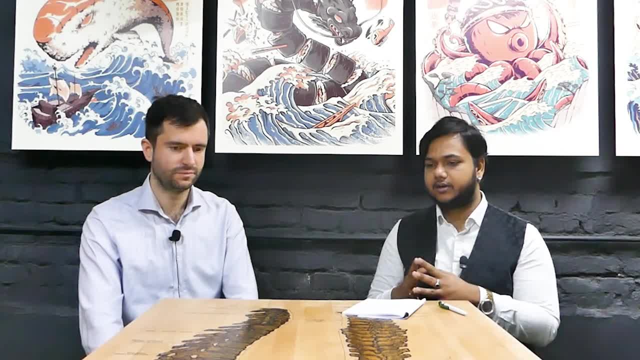 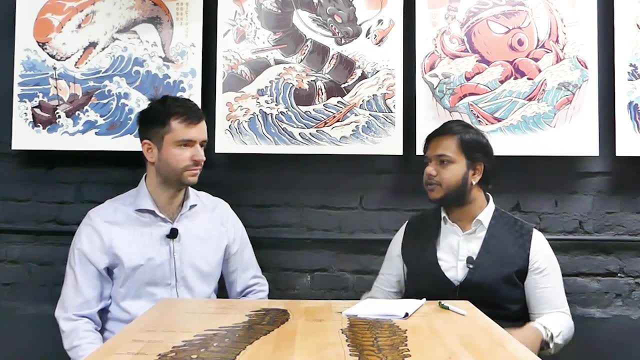 opting for. so, mr peter, give us some insight about, uh, these sort of internships or traineeships that actually guide you, take you through when you're university in university and lands you a job eventually. so, first of all, i would definitely suggest students who are in the final year of 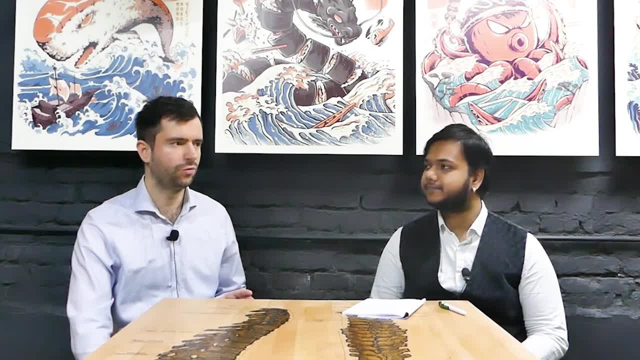 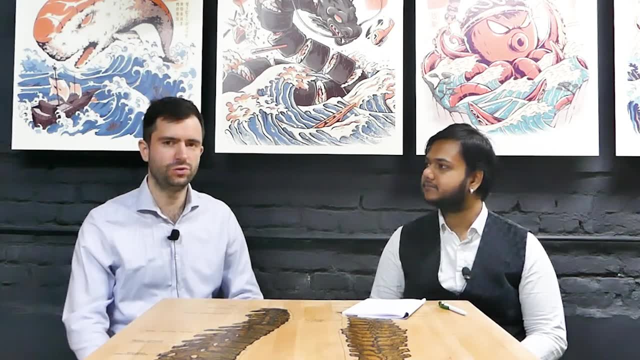 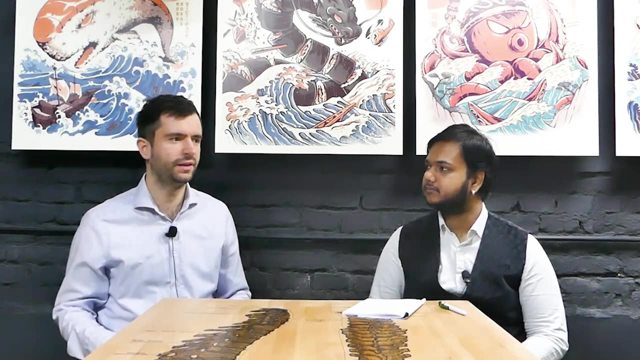 studies. uh, you can also opt for option to. if you select your topic for the bachelor thesis or master thesis, you can also select in which company uh you wish to have. it okay, for example, uh, students can go to various mechanical or economical companies and they can on, on on spots. they can then do some. 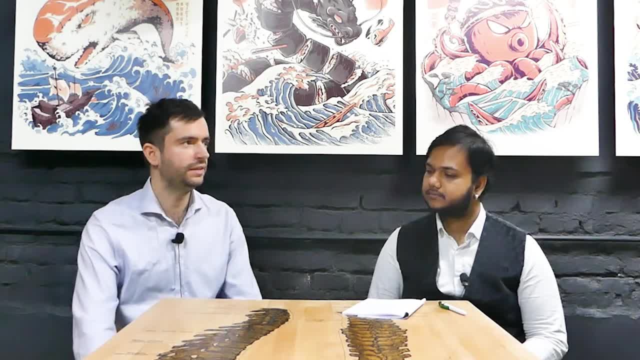 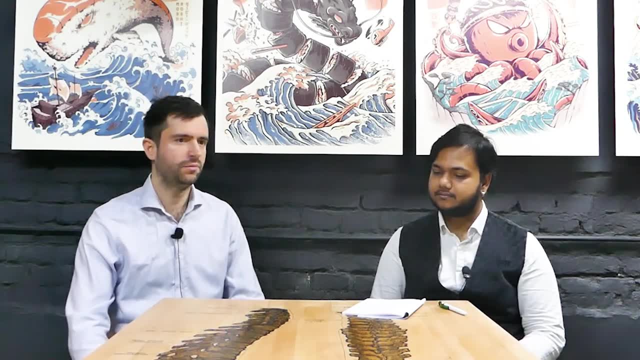 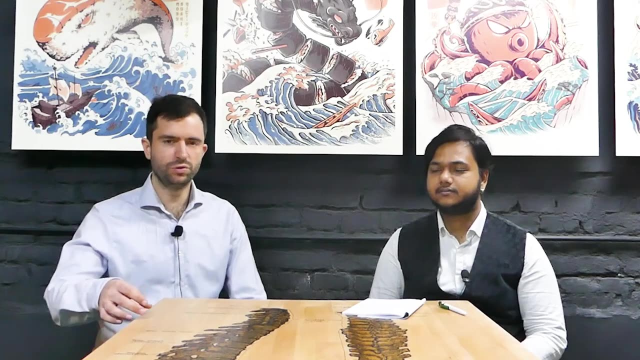 research on in some relevant topic. okay, uh, and even then the local company will see that there is some talented person who can uh, maybe be a collaboration, who can then collaborate with them in the in the future. yeah, so, each faculty of mechanical engineering, automobile engineering or economics, they already have some. 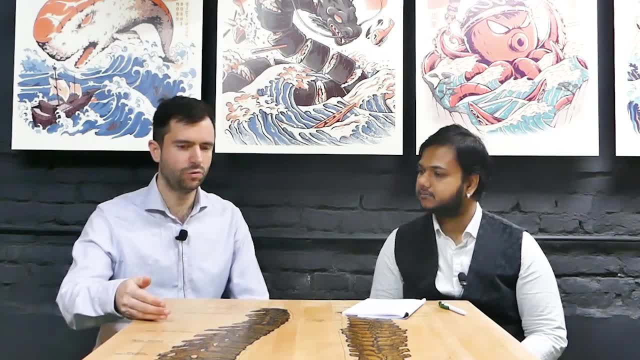 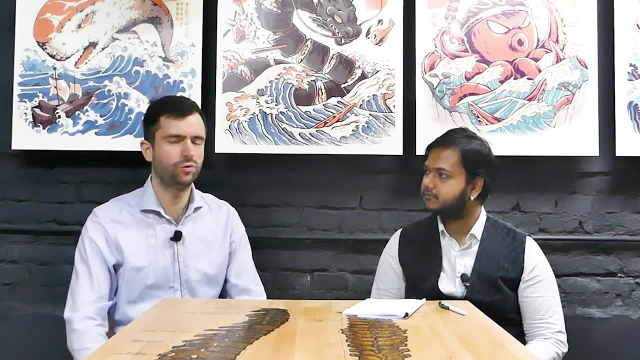 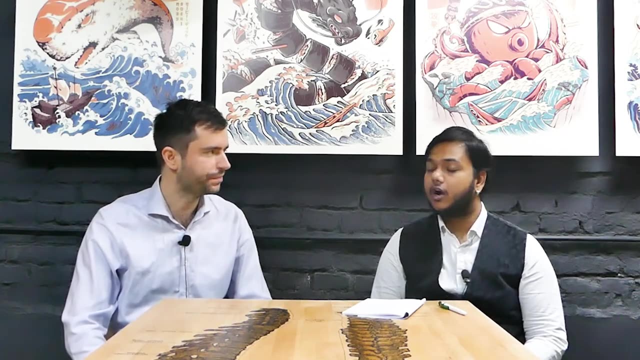 list of partners, and these partners will then give you topics, uh, which they which wish to research? okay, so then, simply, you just reach out to your contact point who is like your thesis? um, this is a supervisor, supervisor, and he will tell you what are your options. okay, that's pretty. 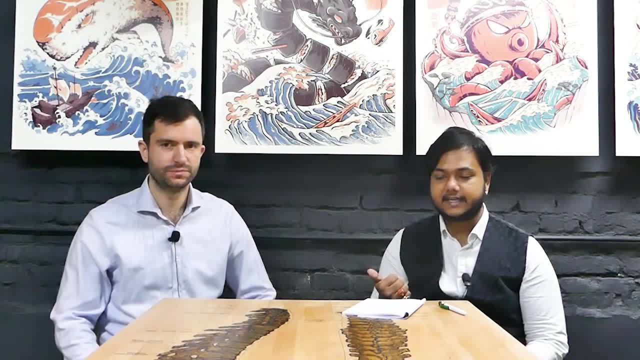 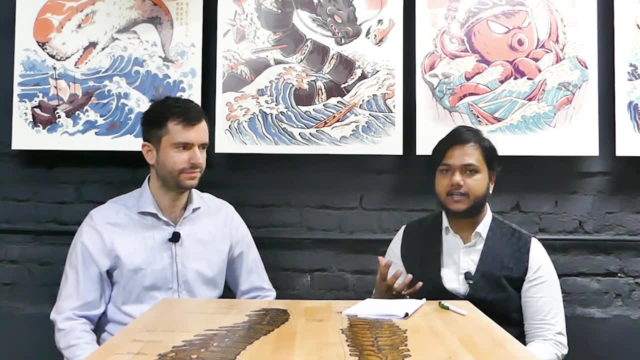 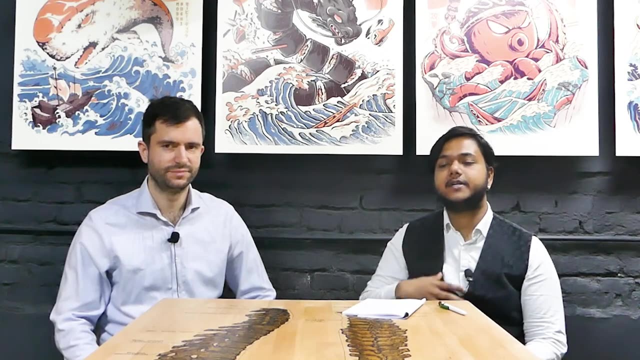 great and this actually opens: firstly, your research is very strong in that case, uh, and secondly, you probably end up with a job after that. there's also a chance that you, when you're studying- i personally did it as well, and many other students did it- so, uh, when you're studying, you might end up in an internship. 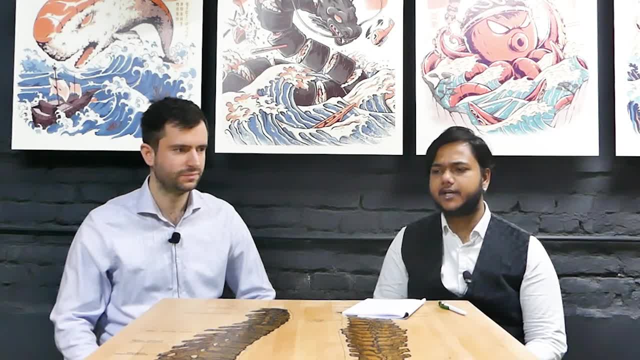 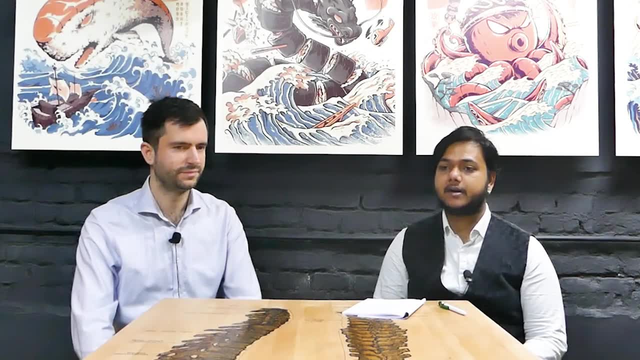 which is relevant to your industry. for example, mr peter is now collaborating and helping many students uh to get like a job in garrett, one of the automobile parts producer here in slovakia- prominent one. so give us some insight how to end up in such sort of a job, how do students find and 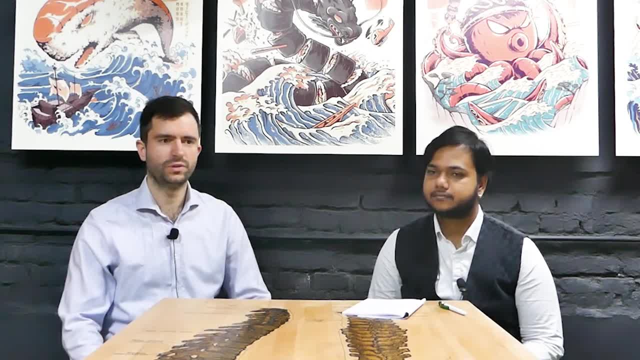 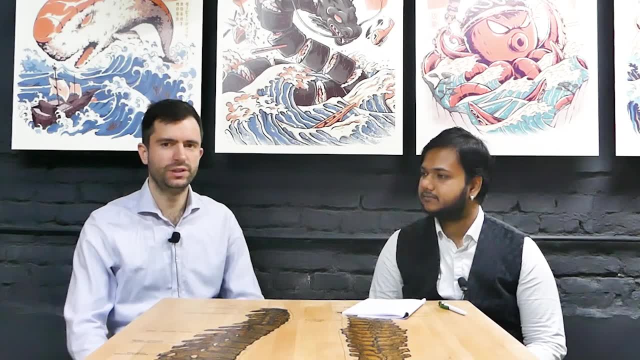 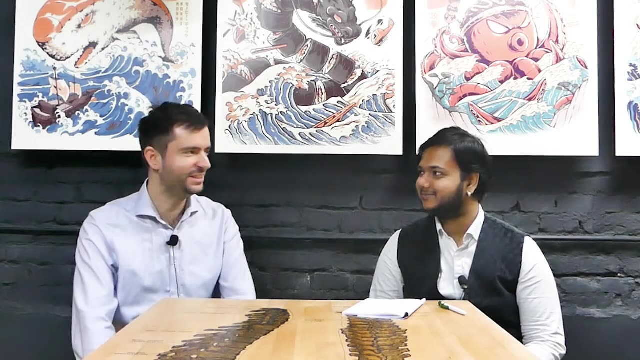 who is the person they should contact regarding the same? yes, so garrett, before it was called honeywell. like there are big uh producers of automobile parts, so in this case, in the factory which we collaborate with uh, they produce store board chargers, or how they call it, tc. 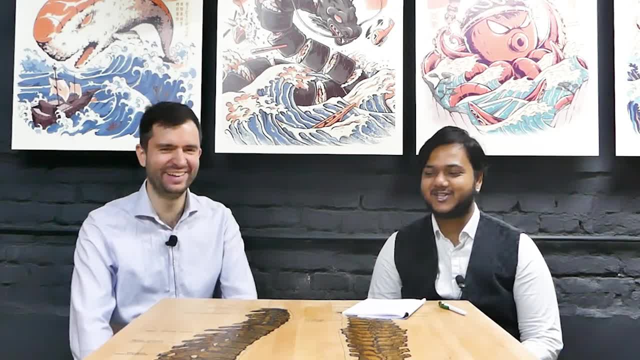 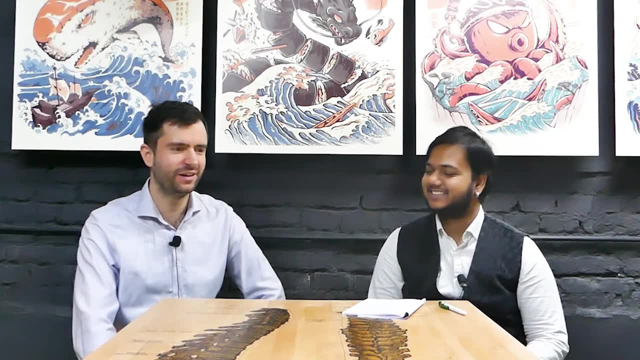 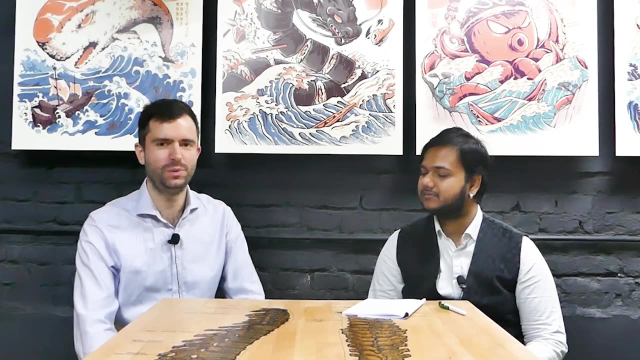 my recent knowledge, if you have seen, fast and furious, that's the thing. turbochargers, yeah, with the nose gas pedal. so basically they do these species for basically any comp, any car. uh, you can, oh, and their procedures are excellent. so it's like not only to get money but also experience. 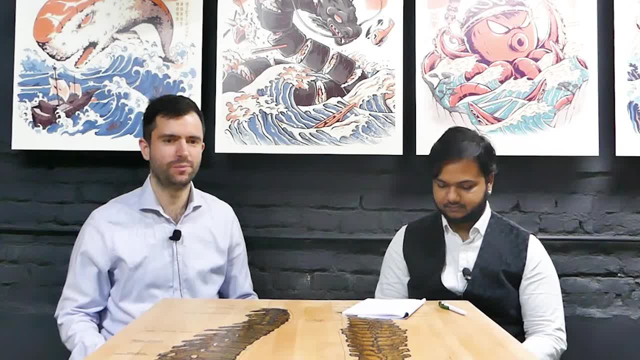 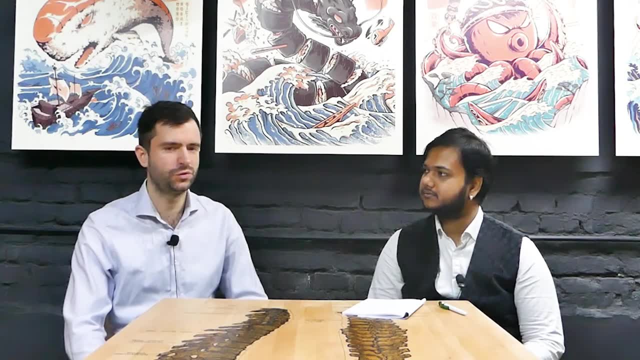 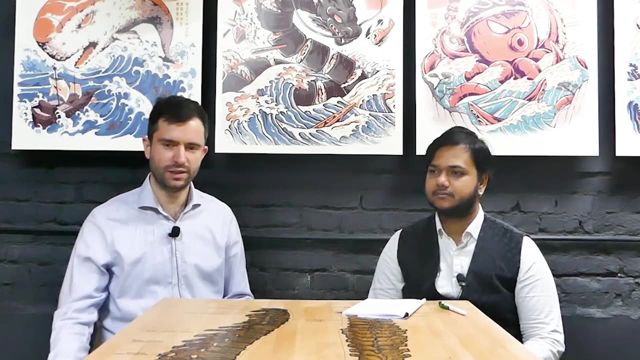 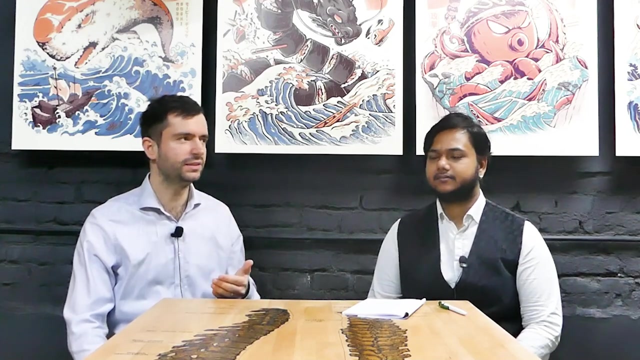 so this uh company, they- we have some connections uh with them via the faculty of mechanical engineering and faculty of manufacturing technologies in its technical university. so they contact us. then we give them a list of students who would like to come for the entry test. okay, and students who pass the test will be then offered place okay. so what you can imagine uh is that you. 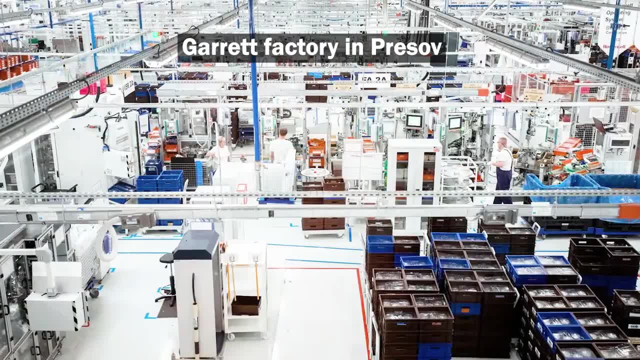 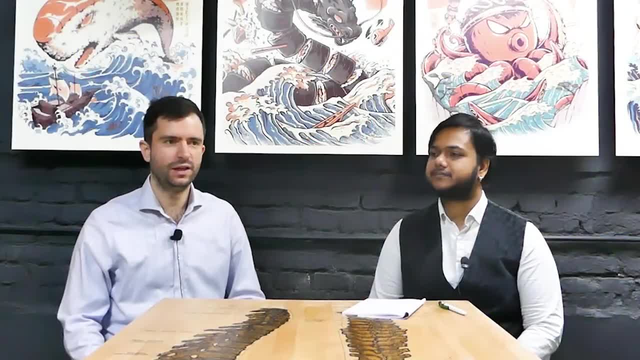 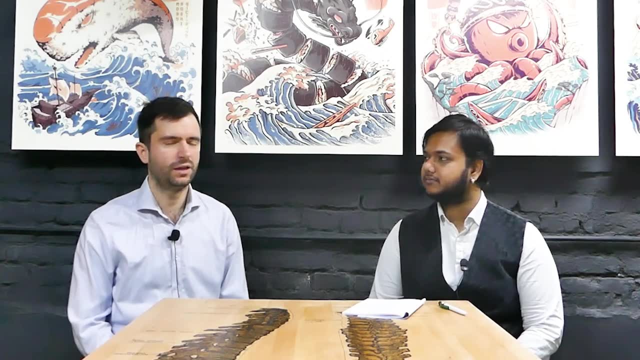 do assembly of the of the turbochargers, or you can do the quality checkups, okay, of this, of these mechanical parts, uh, so there are eight hour shifts and uh, you can then get even the allowance for the food and also some additional payment for traveling generally. this brings me to a question, because people are mostly comparing: like how much? 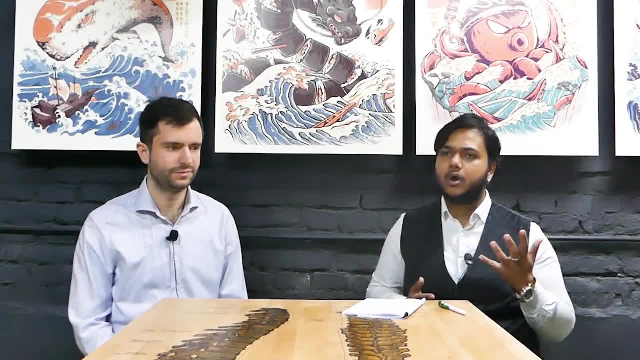 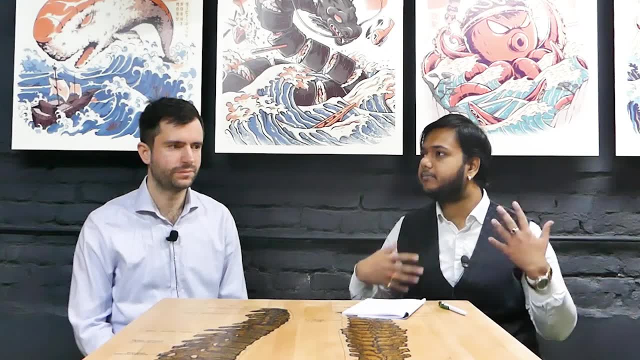 i spend for living expenses versus how much can i make? so what is the generation? you don't have to say the exact number, but what's the approximate number as of 2024? that's like per hour paid not necessarily from garrett, but any relevant job to the industry. 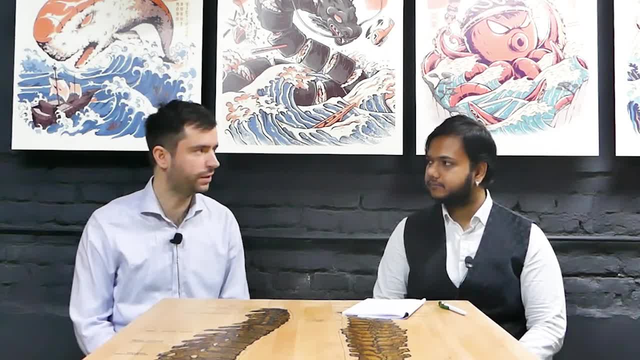 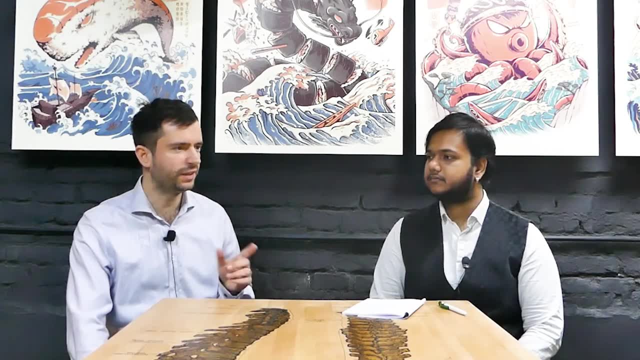 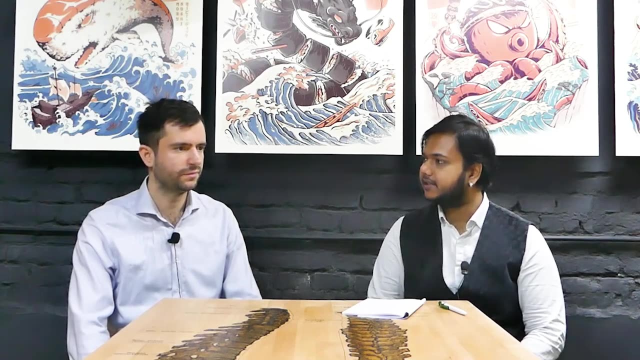 i would say that it would start maybe at four euros per one hour. okay, uh, if you really have some experience in it or, uh, in some specific field like accounting, economics or any of these. It depends from company to company. It can lay up to what scale. 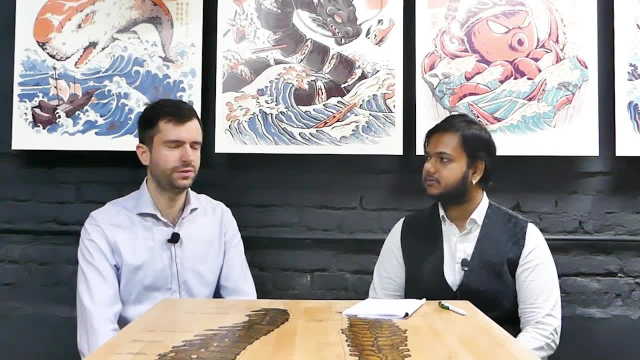 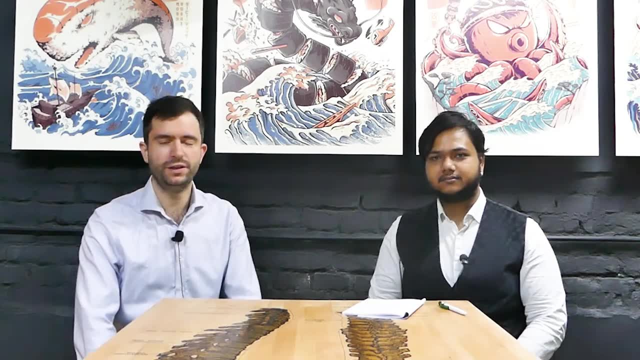 It can okay, In IT it can even be like 20, 30 euros per hour. Yeah, but that's a very typical case. Yeah, But I would say maybe for the starting training positions can be seven, eight euros. 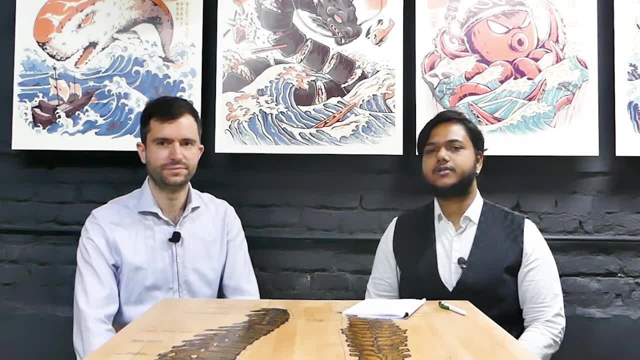 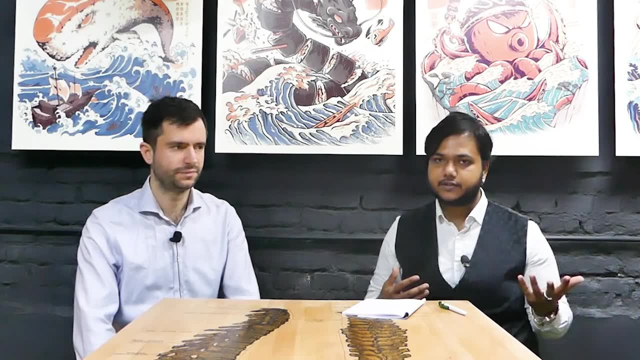 Yeah, seven, eight euros is like a general trend. The other thing is also, we would be actually like giving you insights as of 2024.. That's like how much you can make as well from each of these jobs. So you have some idea how much you can expect from that. 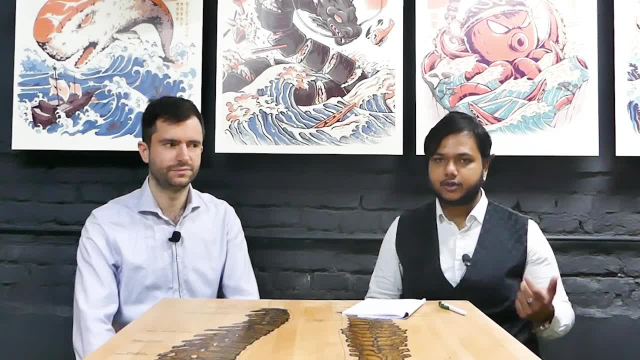 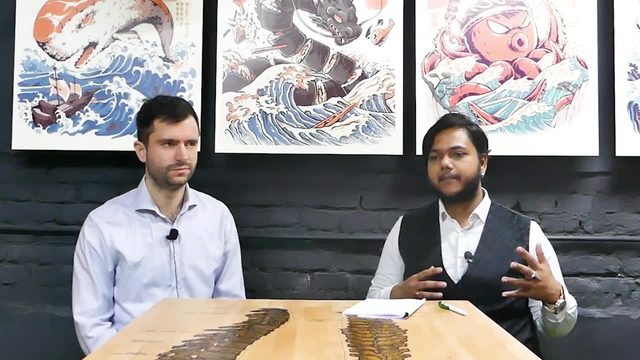 And based on that you can plan your abroad studies. So even from the jobs that we previously mentioned, for example like deliveries and like working in restaurants. So for deliveries in general, per delivery you make in Slovakia about 2.5 to 3 euros. That's per delivery charge. You don't have any gas expenses because you're mostly biking around in the city And in an hour on an average you can do two to four deliveries. So it means somewhat around 5 to 10 euros. So let's say about 6,, 7 is the normal one. The other thing is: how often do you work? So it's completely when you're working in delivery or something like this, it's completely on you. So how often you work depends on that, how much you make. 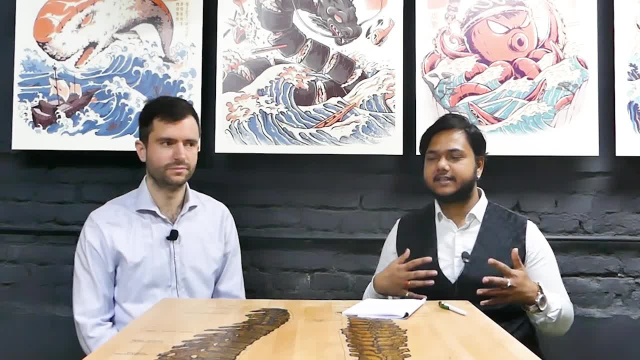 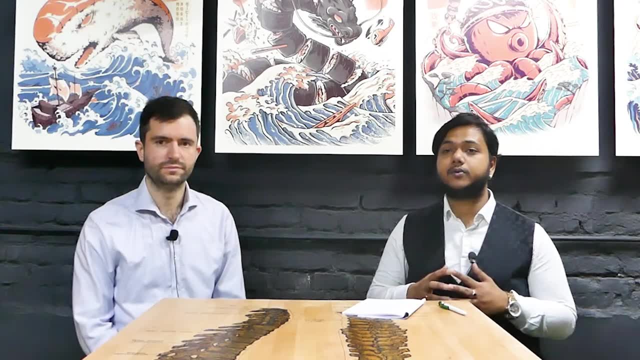 On an average, what we have seen. the people who do like, let's say, every week, few hours just to like meet their expenses- they can make something around like 5, 600 euros. The people who really do it like long hours. 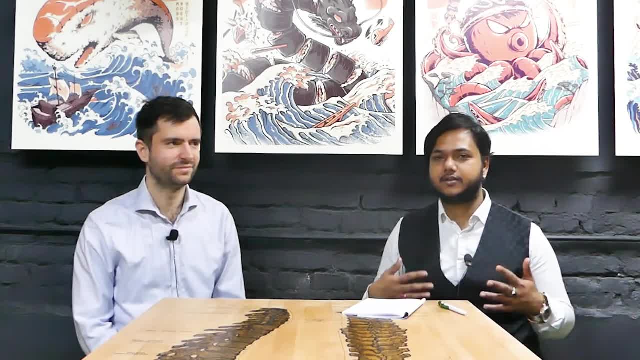 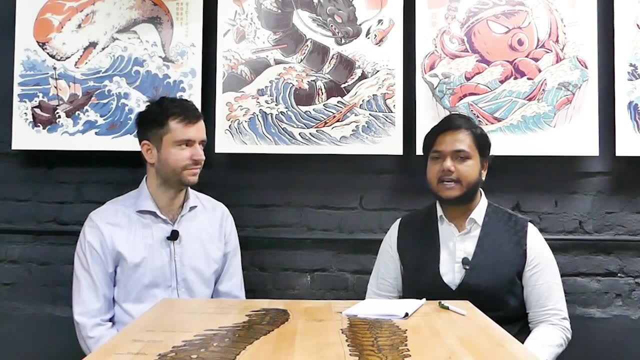 almost every day want to do as much possible. They can even make upwards of 1,500, 1,600 euros as well from the same, And obviously after that there are expenses like insurance and like taxes and all of that. 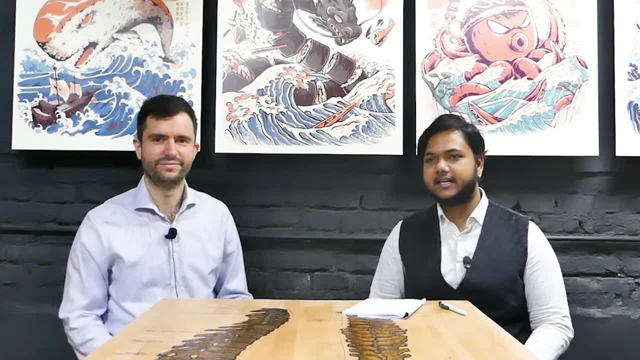 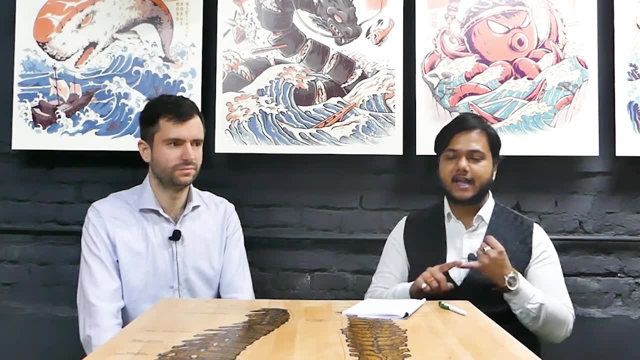 That's apart from this. Then if you're like driving taxis, it can be something. if it's in your own car, you can make something around even 2,000 euros. Then there are expenses like your gas, your car rental. 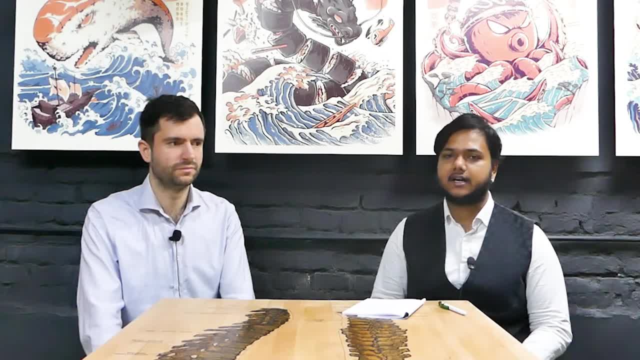 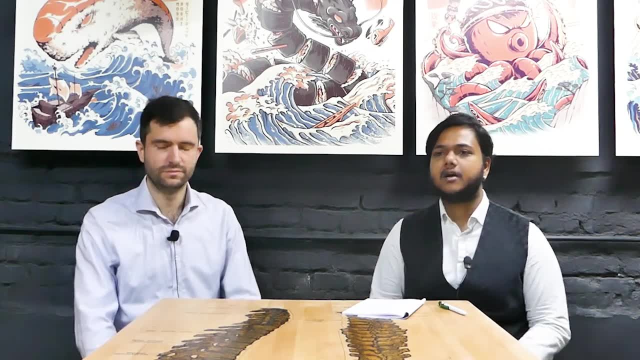 if it's not your car, your car insurance and all of that That are deduced from there, And if you're working in a restaurant, it should be something around a similar range, which is 4,, 5, 6 euros per hour. 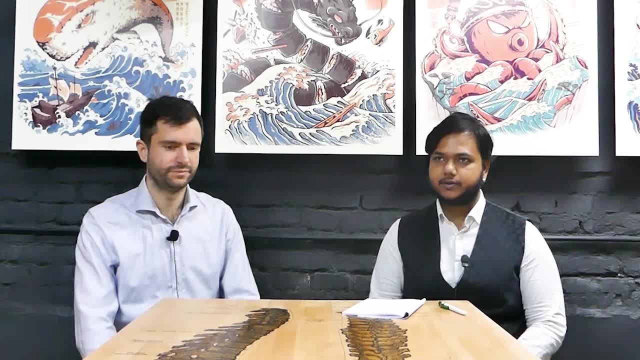 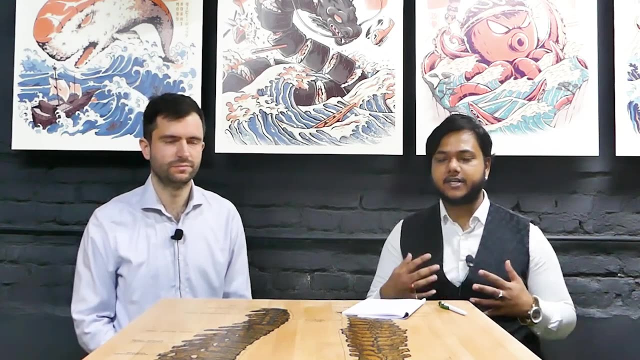 That's the general trend. Another thing, what we wanted to mention as well, and Mr Peter was touching upon, was actually this industry-relevant research and university work. So there are also options that you might end up in apparent internship, which is like, especially if you're in final years of master. 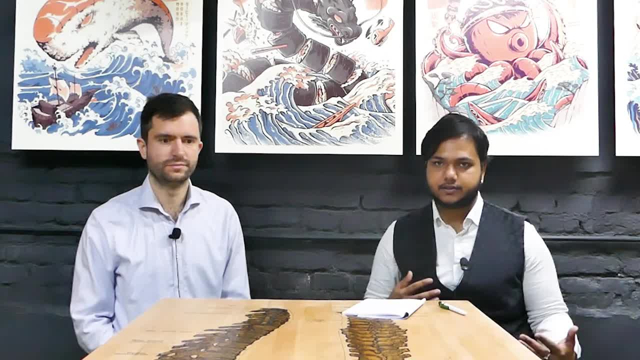 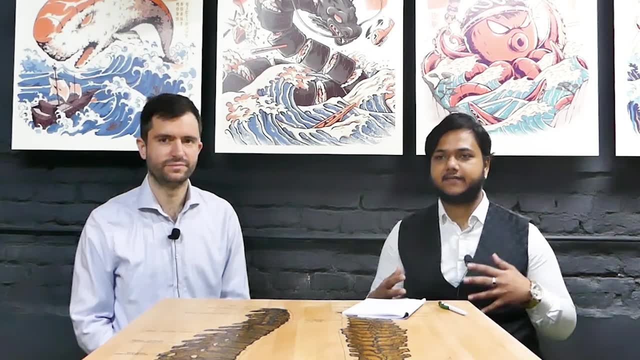 or if you're a PhD student, you might require to give some lectures to like bachelor students or junior students. Or the other option is you might be involved in some research work in the university itself. This pays you as well, something around 5 to 10 euros. 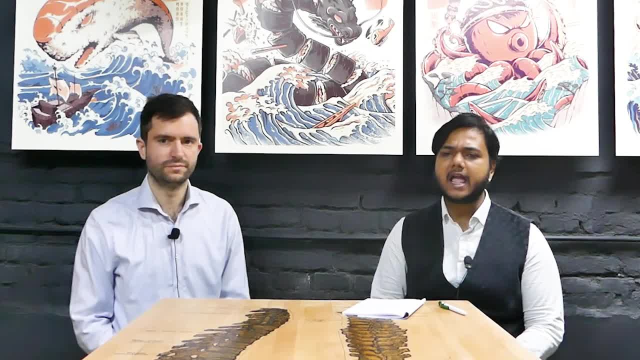 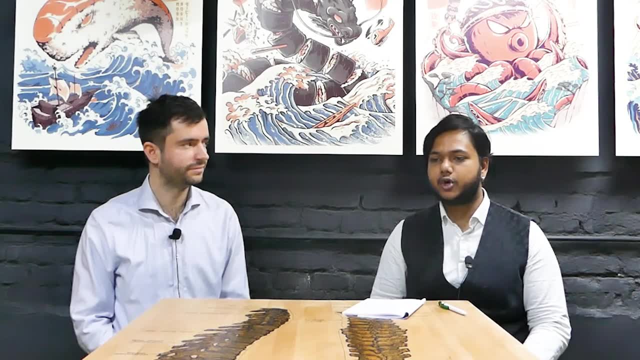 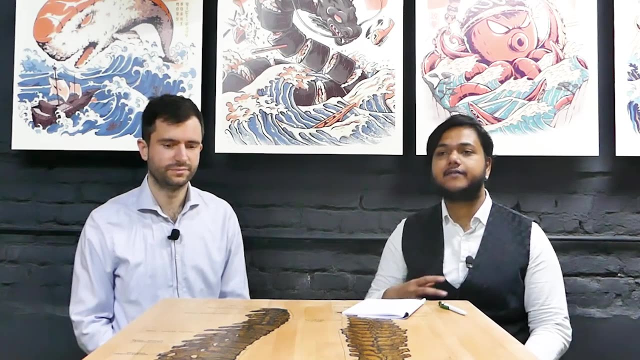 depending on your specialization, depending on the industry And obviously one of the major source from experience. what's like relevant to get a job is to be in good touch with your professors, supervisors and all of the academic staff, because they generally have very good touch. 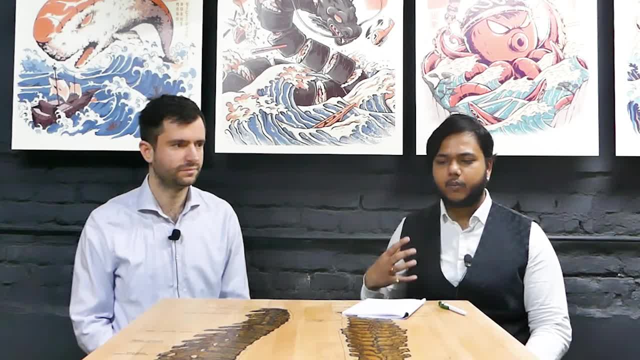 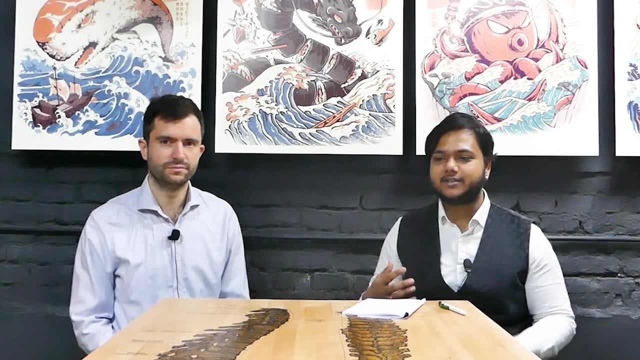 throughout every industry And you know like once you graduate then you're pushing your professor to find you a job or like asking him. this is actually not a good practice. It's better to keep a good relation throughout the study. involve in his research work, show your interest. 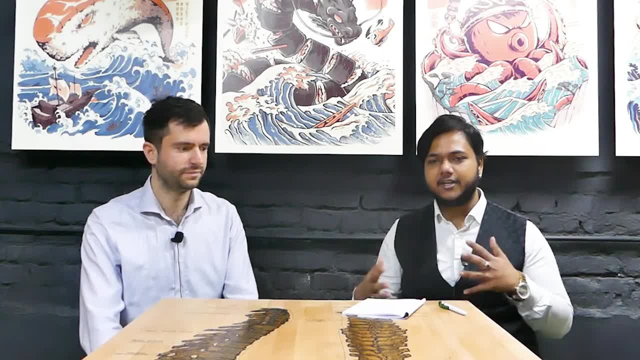 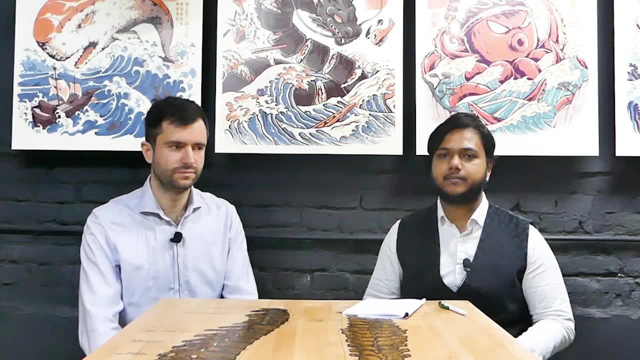 his or her research work, show your interest and everything, And eventually you can ask like okay, I'm looking for some opportunity, Do you have some contacts? And there are many students, many friends I know, who actually ended up in jobs or like part-time work. 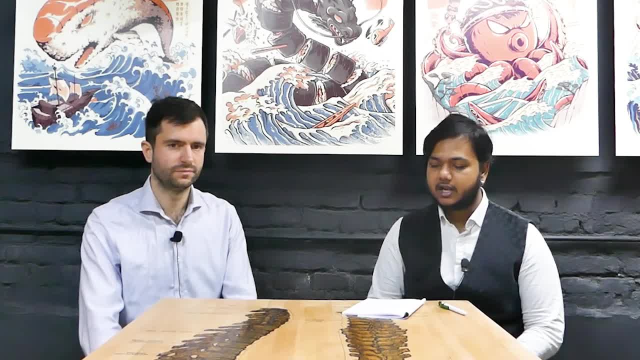 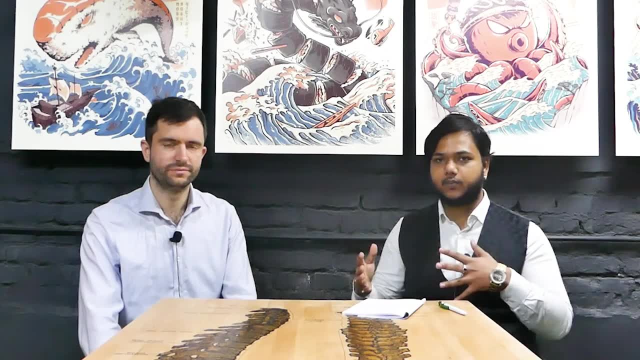 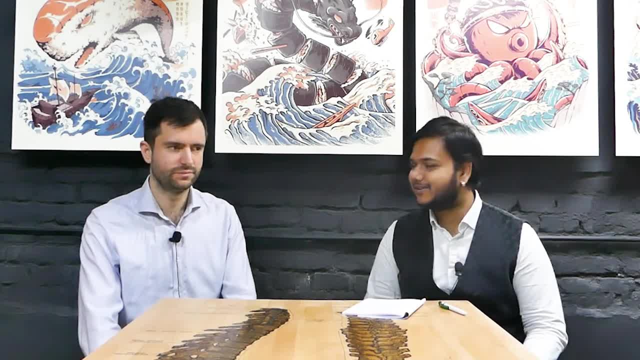 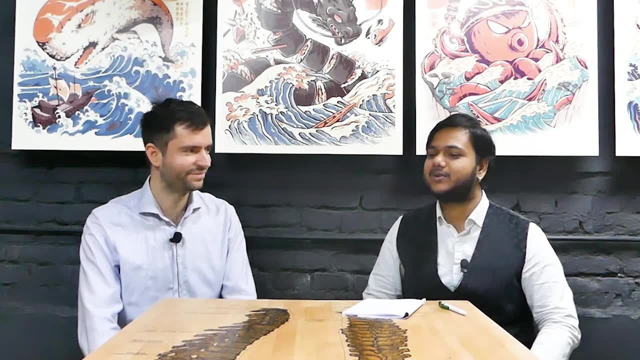 So can you actually like study and work? So, Mr Peter, give us some idea about like: can people actually study after studies? Do they have time? You're like dealing with hundreds of students on a daily level, So do people have time after studies to work? 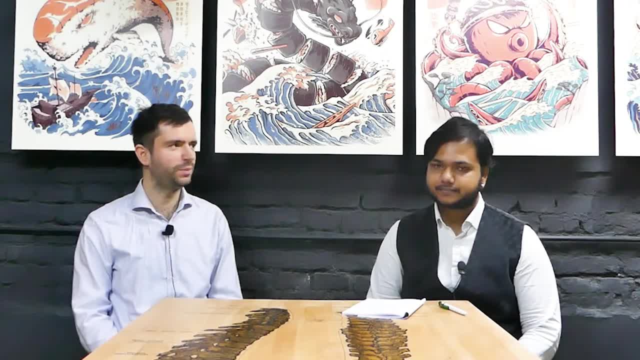 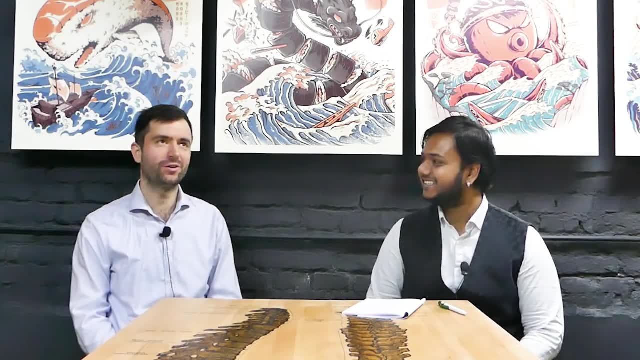 Well, I would say in general answer is yes, it's possible, But specific answer for some study courses I cannot imagine people working Like medicine, Medicine, dentistry, okay, pharmacy maybe no, but veterinary medicine I can imagine. 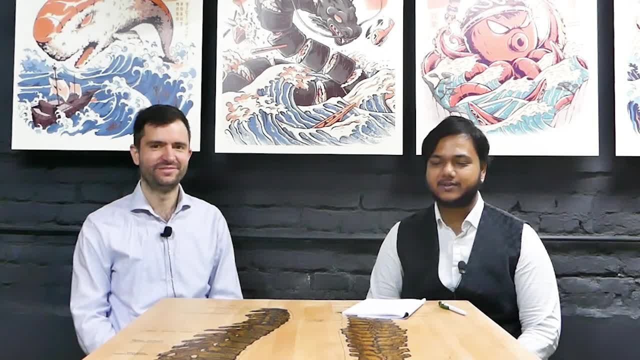 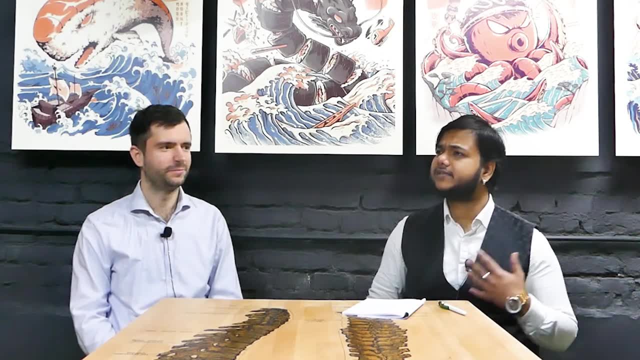 Yeah, these are like really like dedicated courses academically, So you won't have like much time after that. If you do like, hats off to you. But yeah, it's generally like hard. But with other courses which are like engineering, economics- 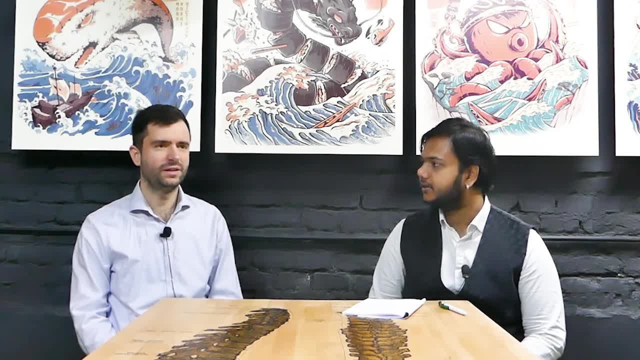 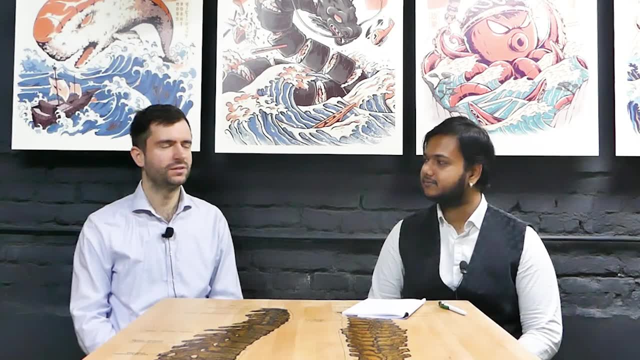 and, you know, like marketing, business and all of this, it should be relevant. Yeah, definitely, Because these technical or economical fields, they are based on more self, you know. independence, Okay, So it means like you maybe have eight to 10 classes a week. 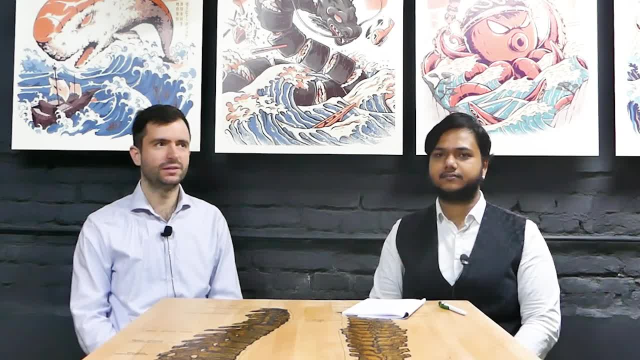 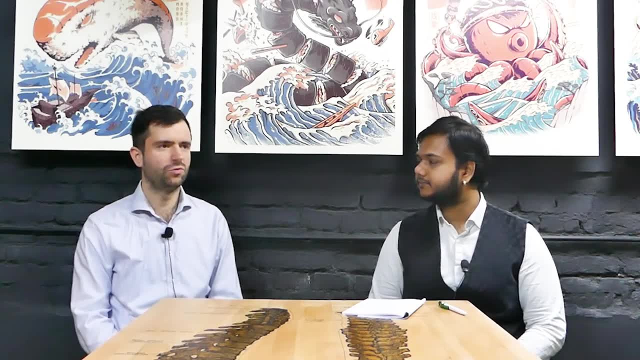 which can maybe opt for 10 to 15 hours, but of the net classes, But on the other hand, you're expected to study on your own also. That's very important. So not only like definitely will cope with that, but like, you also need to take your studies. 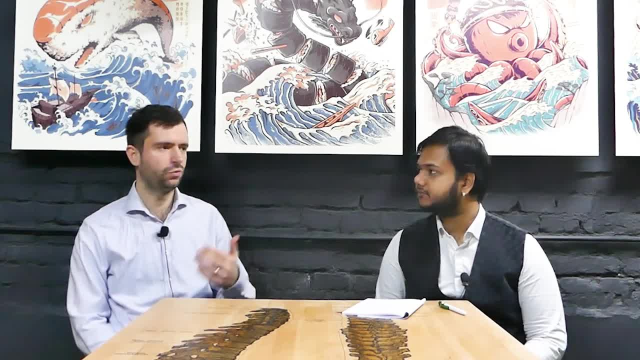 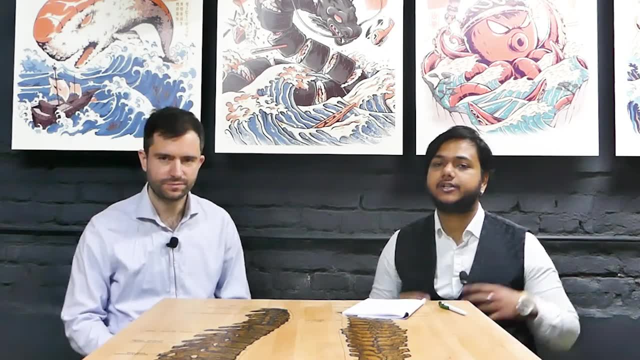 into consideration that we need to pass exam, because if you are expelled, then there are some consequences which you don't wish to face. Oh yeah, because keep in mind one thing: that you're actually coming here as an international student to study, so that needs to be a primary goal, no matter what. 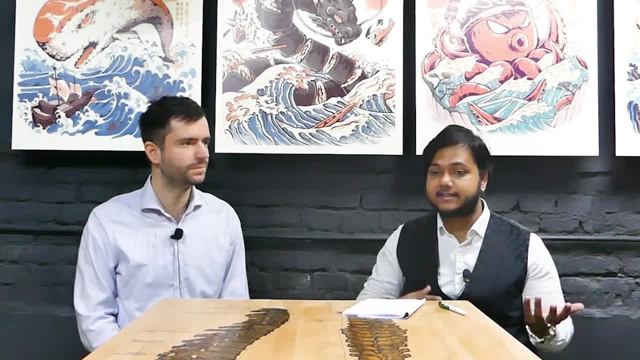 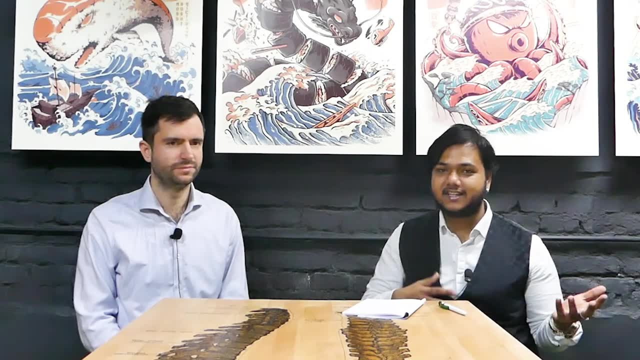 Many times what happens is like students, because they see some money and it's really good money. Obviously it's in euros, So they completely dedicate themselves to some work and then ignore studies and then want to move to work. But the thing is: 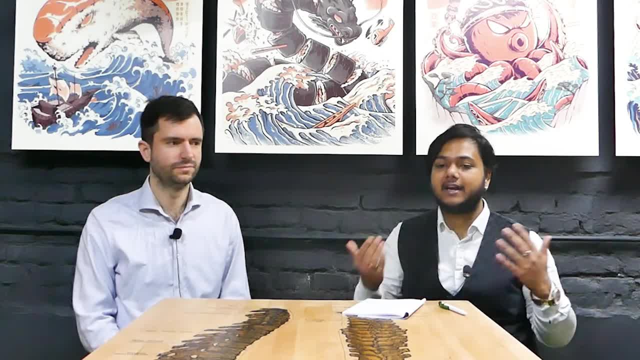 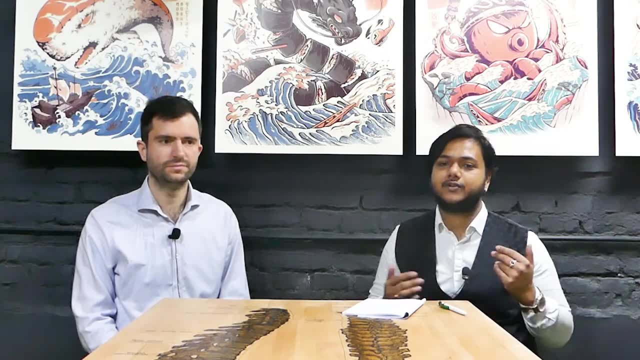 if you don't complete the education you wouldn't have like industry relevant and well being job. For the instantaneous value that's a big part of the industry as well- moment it might look very good money, but for the long run it's not. so it's better you finish your. 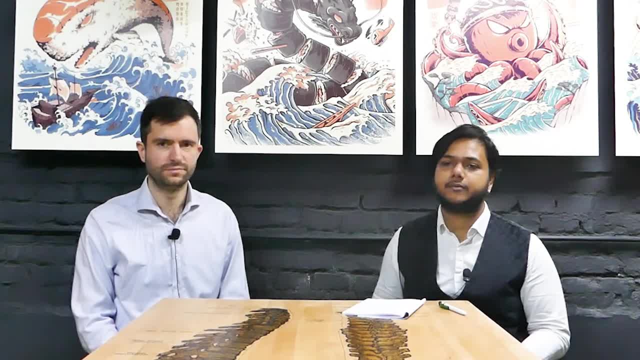 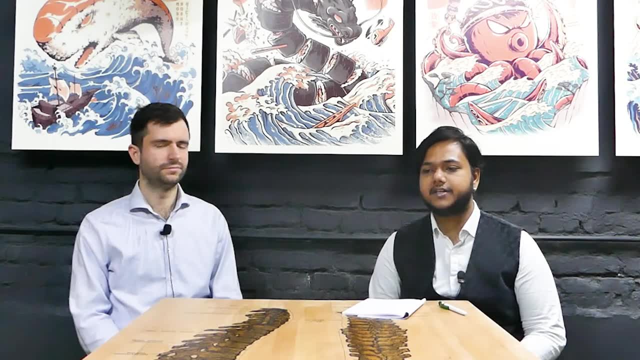 studies in the meantime, get experience and then move to like some full-time good jobs. that should be a good practice in general and what we see, or when i was a student as well. the general trend is you work somewhat from like monday to you study from monday to thursday. 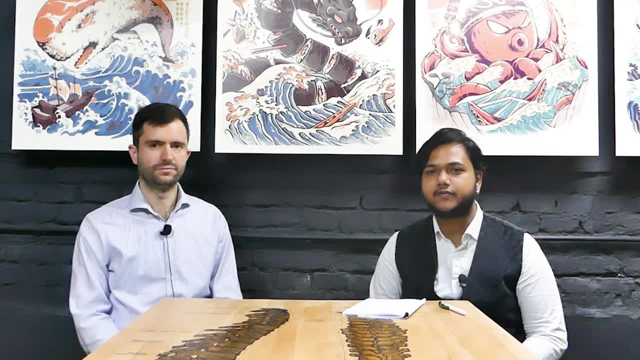 fridays you have generally like some optional subjects or physical education or something like this, so you can say friday, saturday, sunday, you're mostly free, and definitely evenings. you are free in the general universities and general courses, so you should be available in the evening to work. 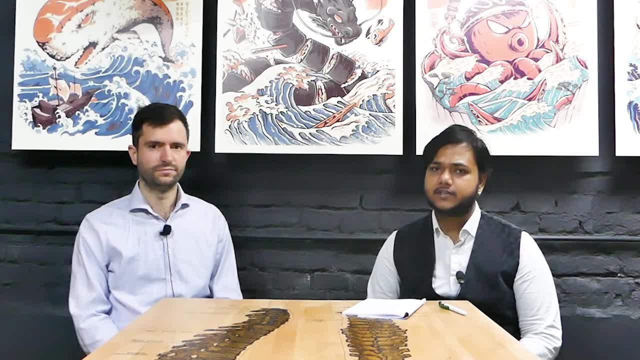 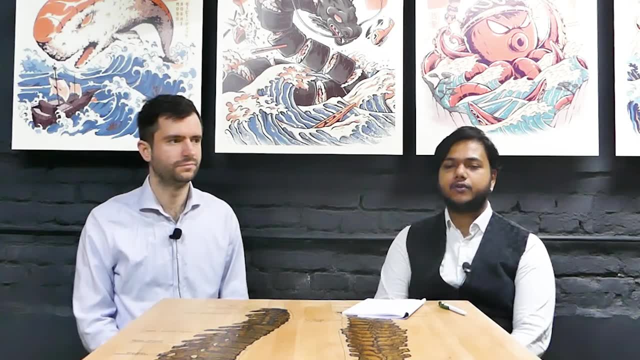 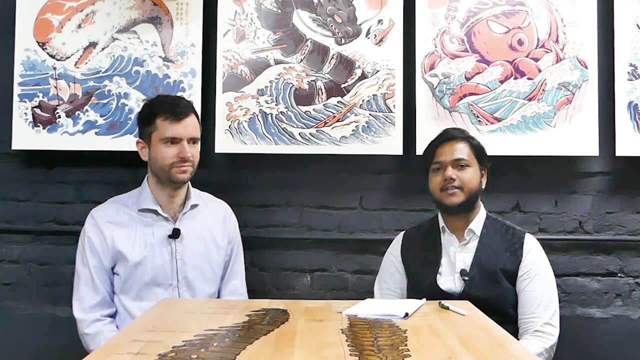 you should be available during the weekend to work depends on where you find your your opportunity. we had a few friends also. we will link a video to viraj, one of our close friends. he was studying from monday to thursday in koshetse and was traveling five hours. 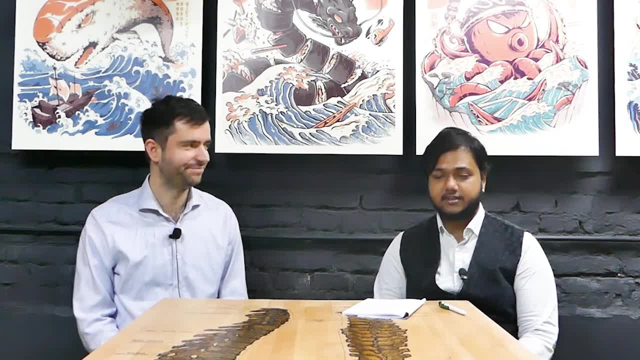 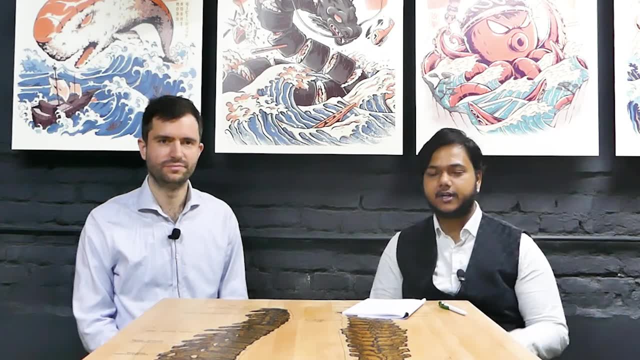 by train to bratislava to work during the weekend, and that is. many people do that because maybe they have more relevant opportunities there. but yeah, you can work in bratislava, you can work in koshetse, wherever you find more relevant opportunities. nowadays, what's also prominent and coming up: 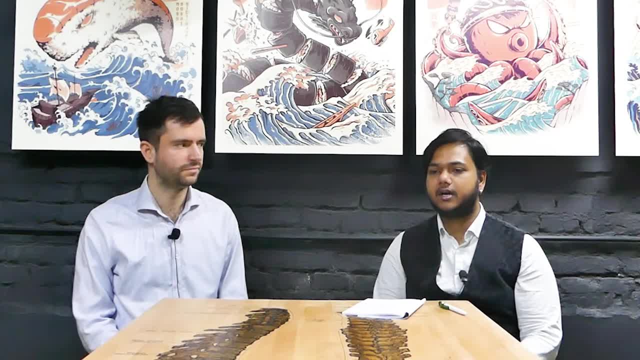 is like home office. so if you have like some experience before coming to slovakia, you might also find some home of office relevant opportunities as well. and how do you see like the scope of work after you're done with your studies and what do you see like the scope of work after you're done with? 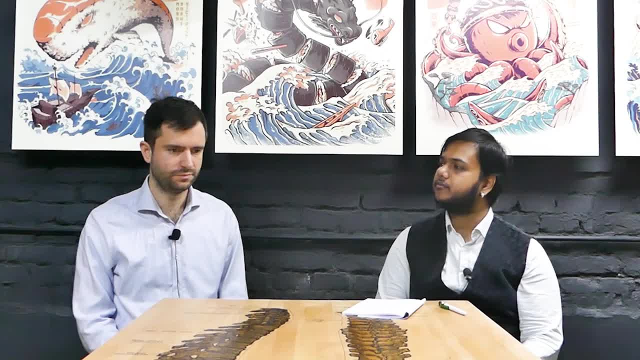 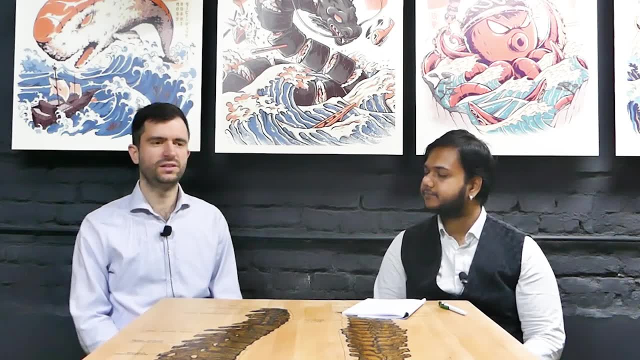 after, like, they finish some uh university? do you see like people have more chances of getting a or landing in a job after uh if they have some internships? yeah, definitely, i can see currently there's like big demand for qualified workers, like both qualified and unqualified, especially. 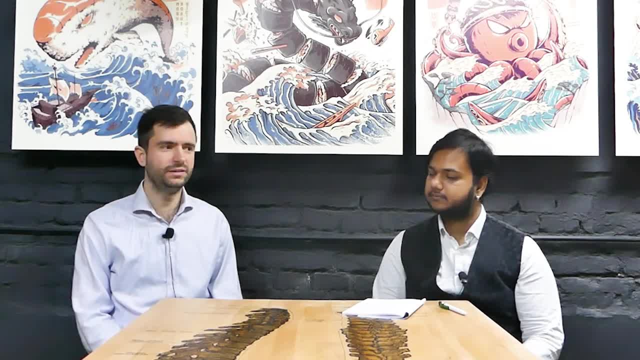 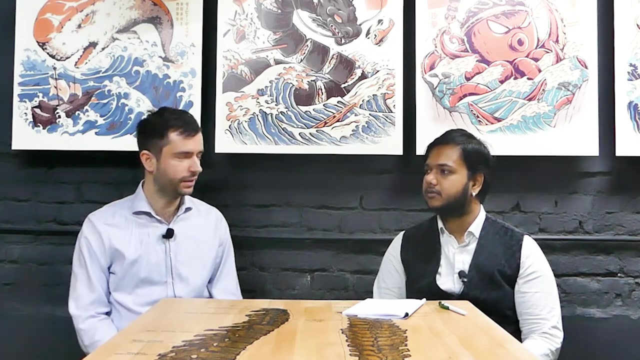 in technical fields, so definitely in it. that's uh very easy to get. then in mechanical uh, there are like multiple companies that give uh even to english speakers uh jobs. i can make them named Segula in Bratislava and then this garage. they also told me that they will start hiring. 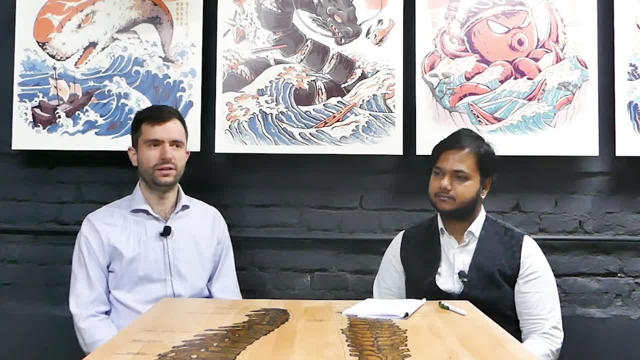 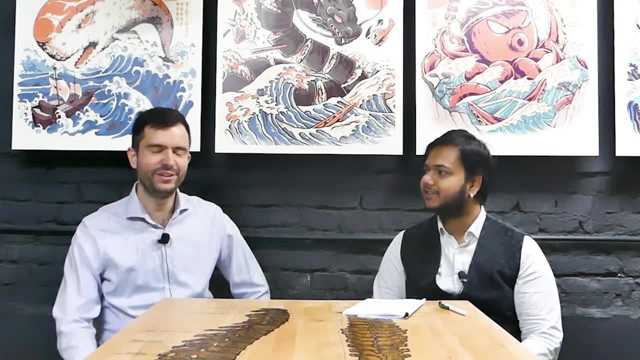 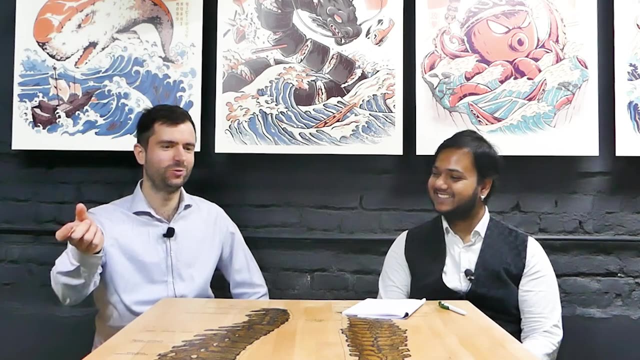 english-speaking graduates. so then there are some indians who work in Peugeot, Volkswagen, so then also Land Rover, Jaguar. exactly that was my, that was my idea, because it's an indian company, you know. so basically the workers who it's inter intra company, it's for a company shift, so i think 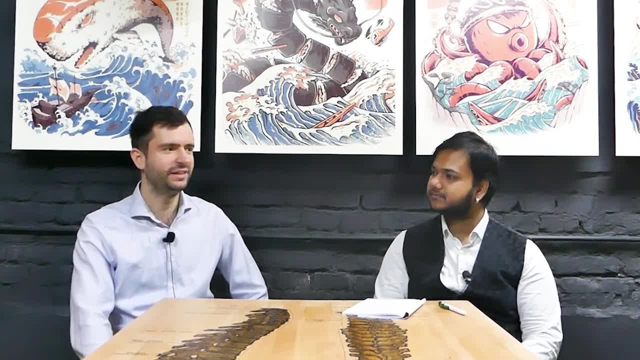 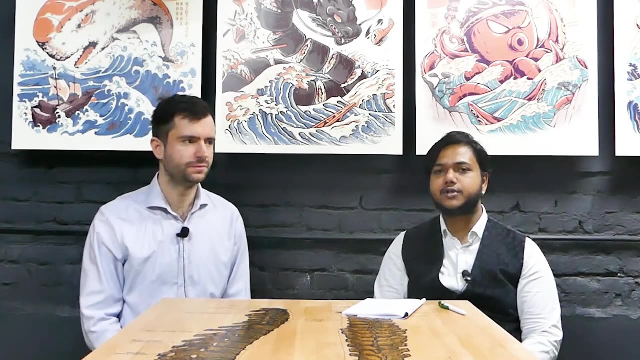 200, 250 workers are now in in uh, in um, it's india also. no, uh, yes, it's india. so and there is obviously like automobile in general is a very large field and it is very growing field in uh, so i guess. so these two um industries, you should uh find relevant job opportunities. so like uh, or really. 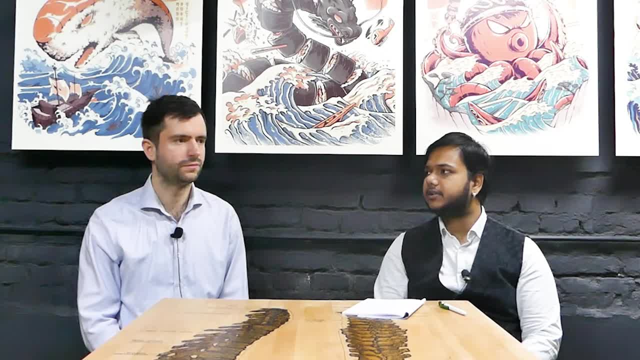 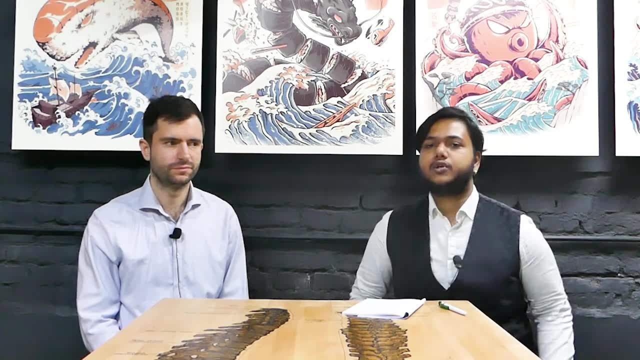 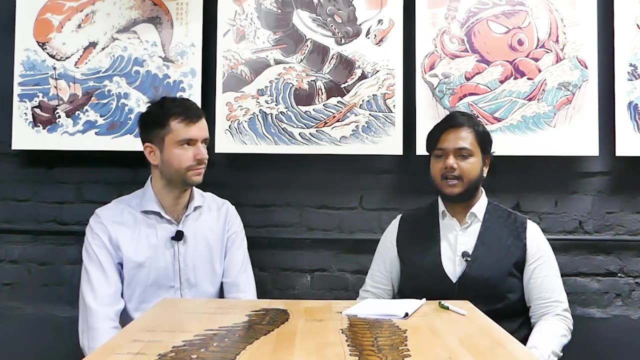 these two industries. there is continental tire company, for example, and several. we have some videos. we will link it also to segula with the hr there, with the country manager there, to they explain, like, how the recruitment process goes, what are the requirements and all of these details regarding it. and, yeah, also you, we have some personal contact of theirs over there. so 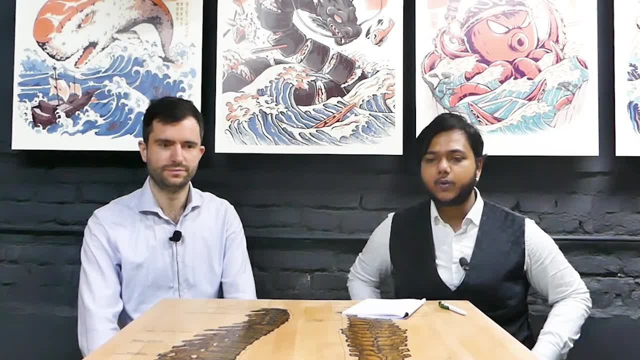 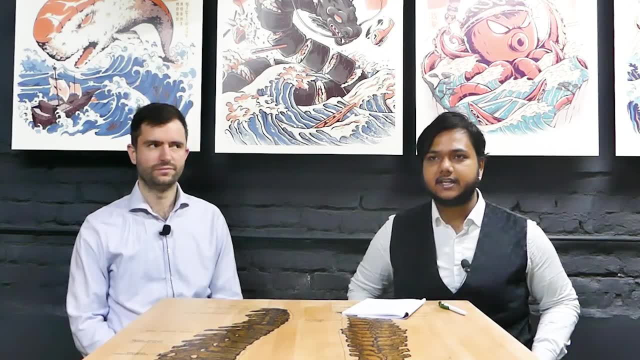 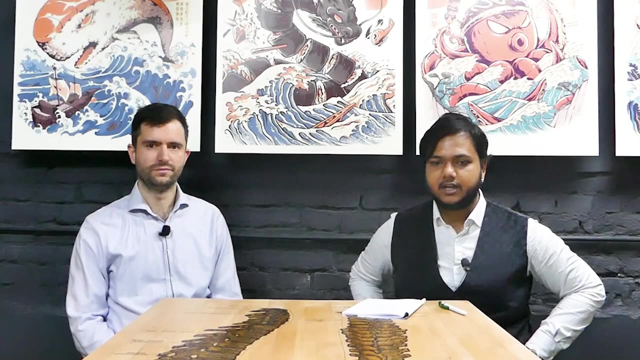 you can actually personally reach out to their personal email and write them, send them your cv. so do check out that video as well. uh, and in general, if you are like at university- as someone who started at university, uh, i can suggest you is when you're at the final year of university, um, when you're actually in the initial years, try to get at least. 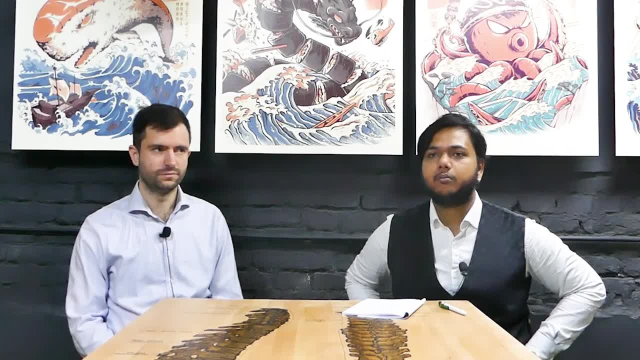 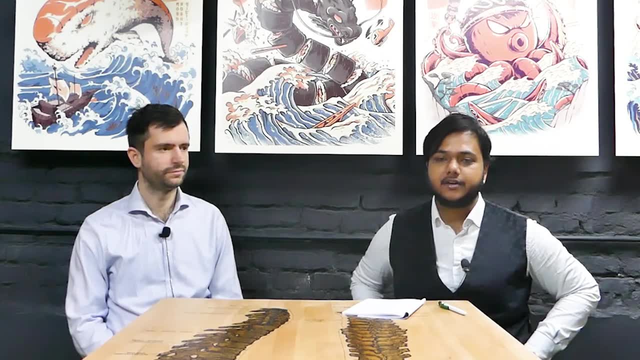 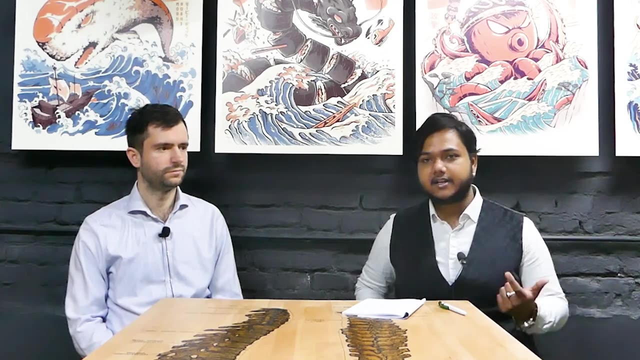 one internship or one relevant doesn't matter about the payment. more focus on the experience that you can get from there- the experience certificate. that's very relevant and important. and when you're in the final year of university, do look for internships and traineeships and graduate programs. there are several. 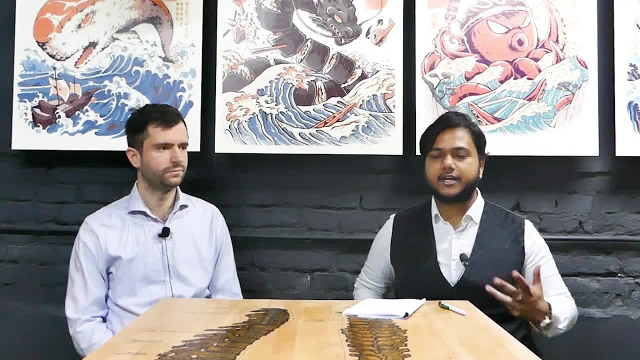 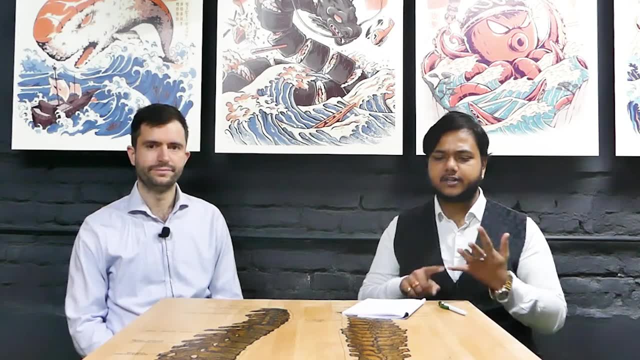 companies in slovakia and all over in europe that offer graduate programs. this is generally from six months before you graduate to six months after your graduate. that's like the eligibility criteria. procter and graham bill um, swiss re uh dell. all of these companies, even amazon, are offering these. 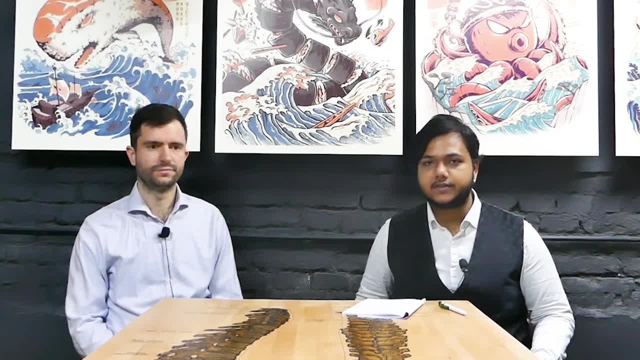 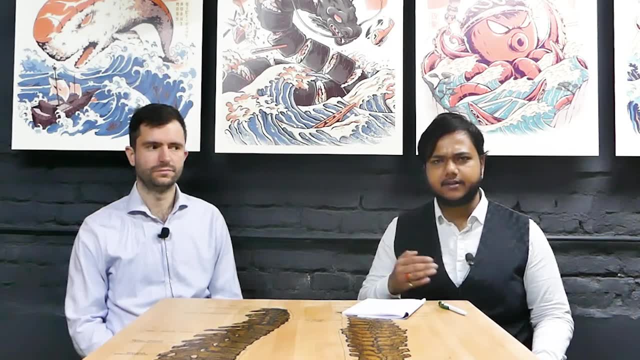 graduate programs, and this is generally for one to two years duration, where you work in multiple departments. then you realize which particular department you like and you have a good salary anyway. the salary is pretty standard. so then after that you have a more relevant uh industry and you grow from there. so it's a very 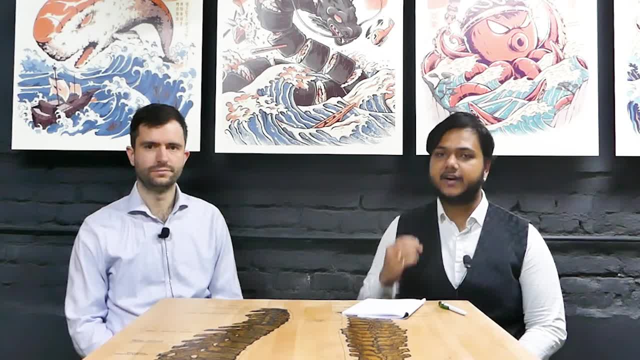 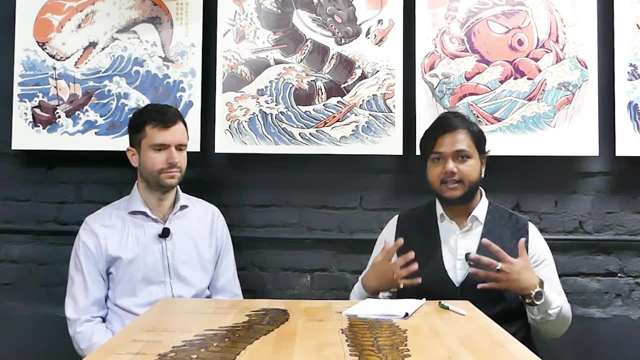 good pathway. but, to be specific, these are very competitive. so there are obviously, like the local candidates, there are candidates with like uh language, uh abilities that they might be specialized in uh in europe. so if you're only speaking english, it might be very competitive for you. but the good. 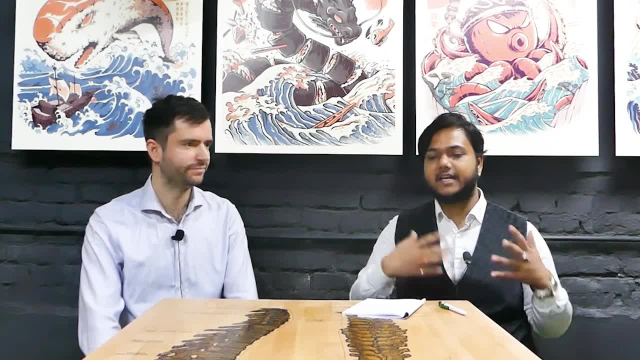 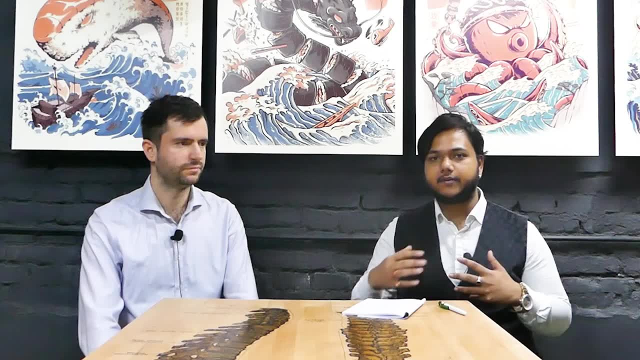 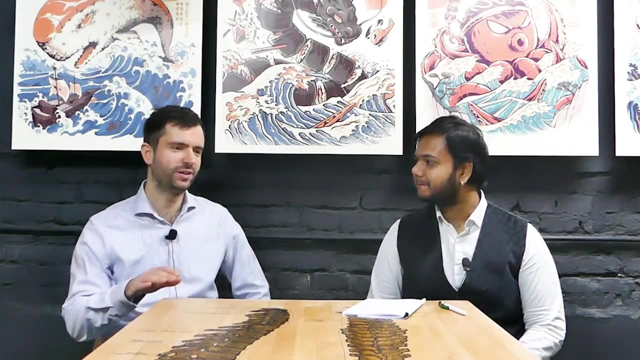 part is you need to uh like the catches. you should apply to as many um opportunities as possible, because if you can end up with in one of the graduate programs, uh, the career prospect from there is really good. oh, okay, maybe here i will uh ask question. sure, because you mentioned like it's really competitive. 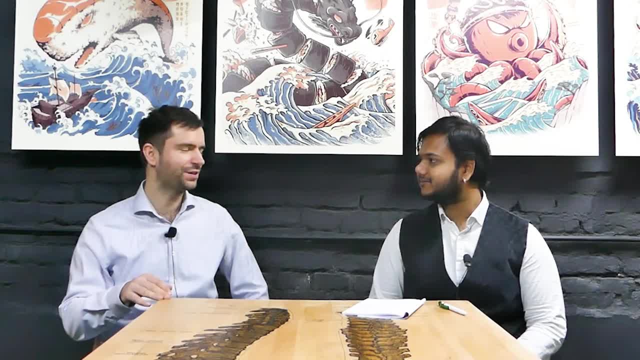 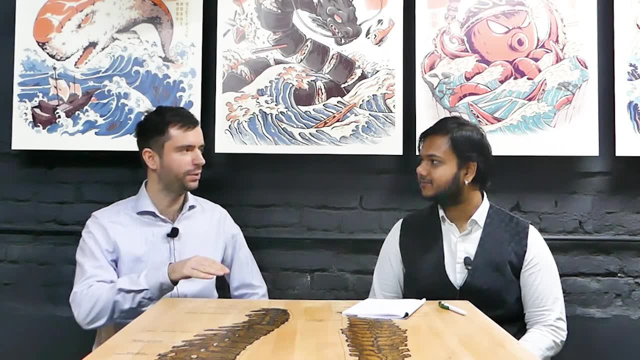 so when we speak, maybe, uh, if we speak in numbers, what do you consider to be competitive in? like, how many applicants would you find competitive in slovakia companies? how many will you find in indian companies? okay, so that is something you really cannot uh like compare. i'll tell you the reason. 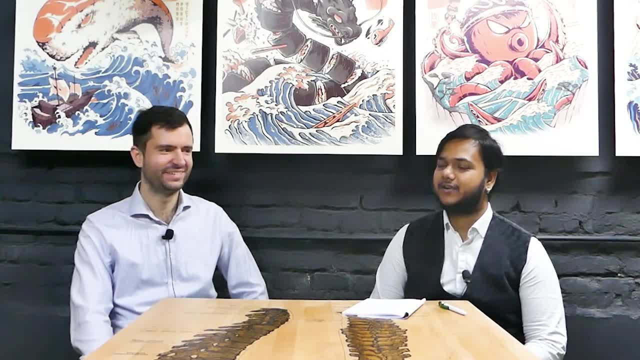 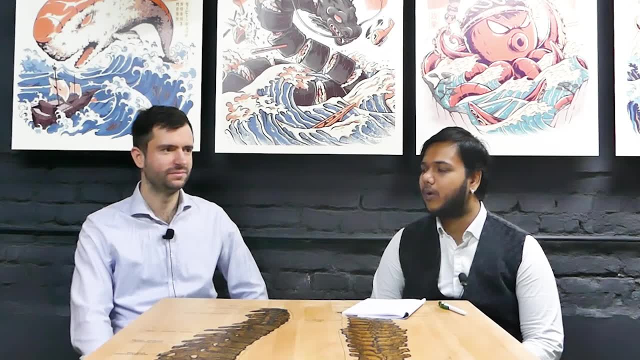 okay, there are a few reasons. firstly, in india, like for, let's say, graduate uh position or something, uh, there might be like thousands, like literally thousands, maybe five thousand applicants for one particular position and there might be, like you know, the uh two people like taking in that position of five. the ratio is much, uh, you know. 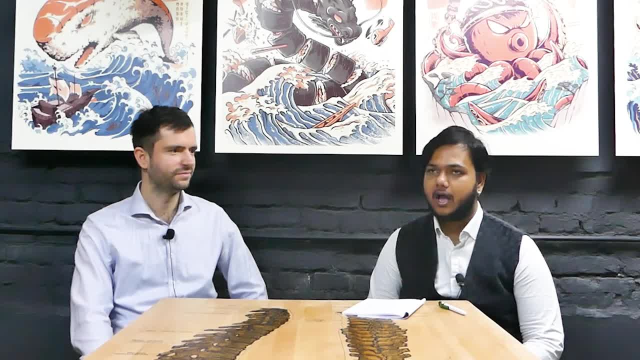 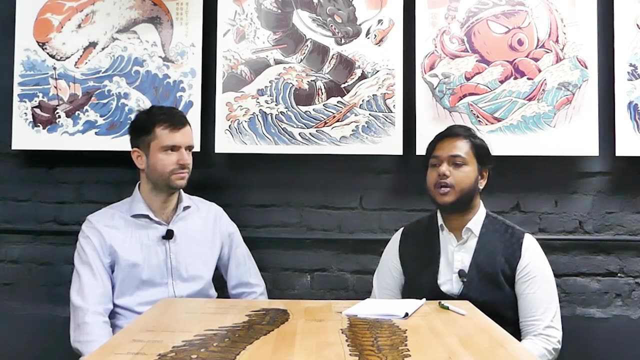 much different, but in slovakia, for the same uh, let's say uh position, there might be like 200 applicants and two are taken. but there is a difference over there that if you're a non-european candidate, you don't have hold a european passport and you don't speak the local language. so there is. 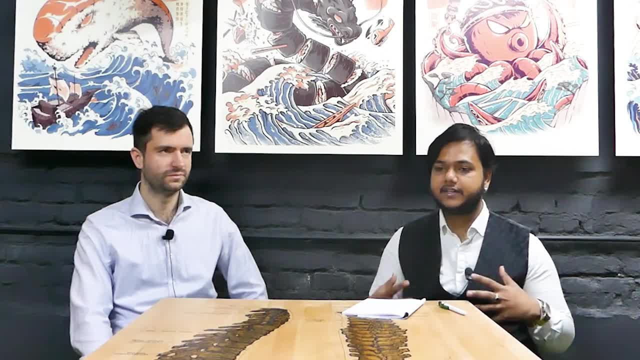 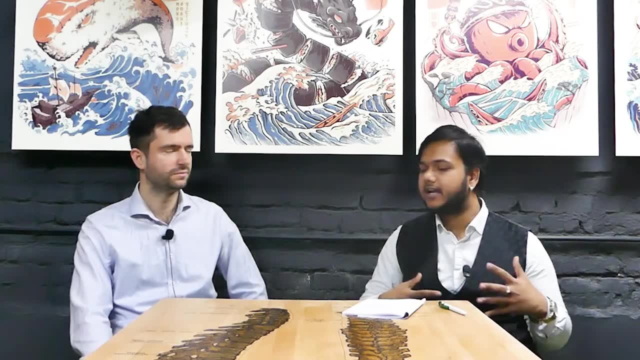 like, uh, more priority given because of the language and everything directly to, uh, the local candidate at first, and also because of the work permit and the visa process and everything around it, it's more priority given to someone local and then the priority is given to you, so you have to. 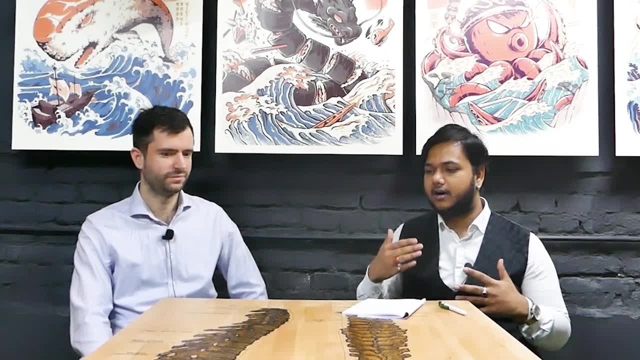 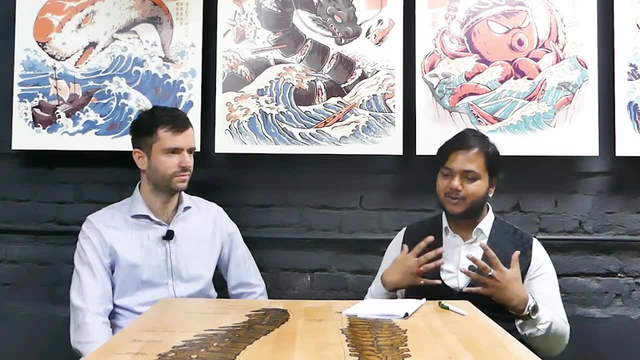 already believe it- that your application is, you know, ranked a little lower because you don't have the language, local language or multiple language abilities. firstly, because in europe people mostly speak multiple languages, not only one. that's the first thing, and the second thing is you don't hold 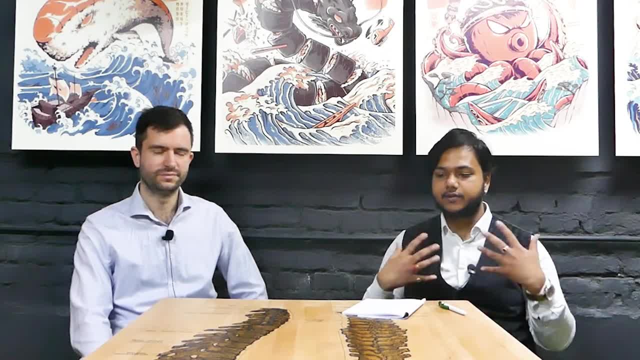 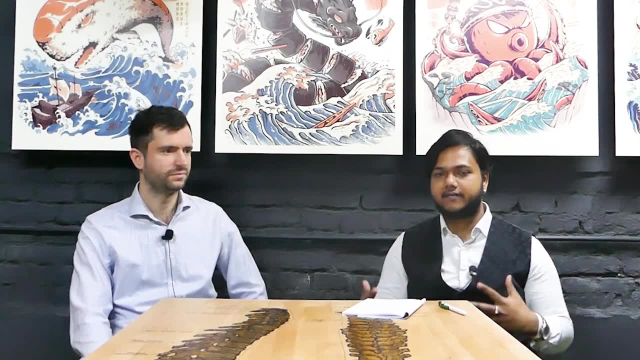 a passport, so it means the company that hires you or gives you the sponsorship they have to do a full visa process which might take, like some other three to six months long process to change your residence card and everything, and this is something that the hrs are very concerned about in general. 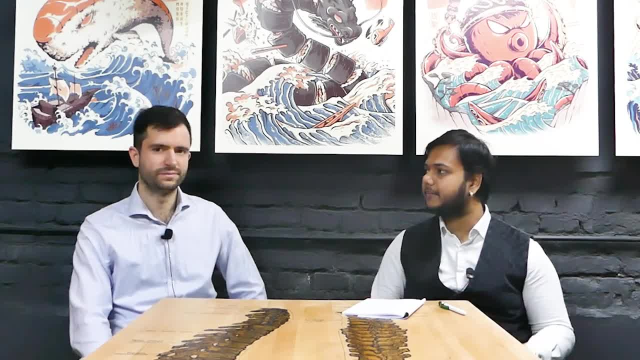 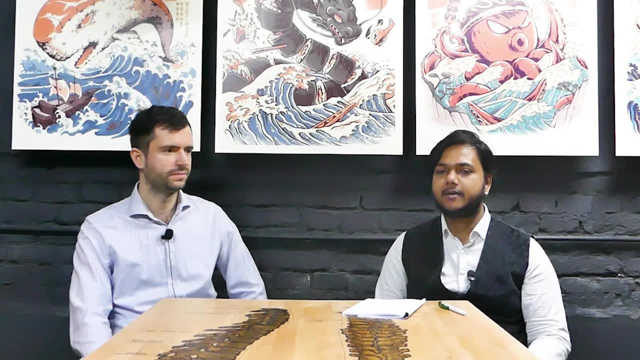 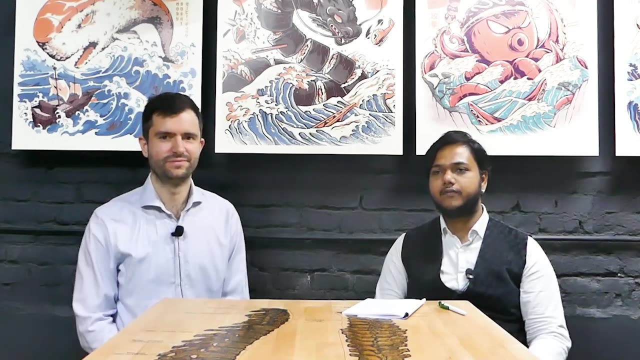 you so. so for that reason it is competitive, uh, as an international student, uh, but yeah, uh, the best is if you can have a recommendation- and recommendations are possible from people like uh, mr peter, uh for uh, from professors, from someone, uh, you know from university who you can have a good touch with. 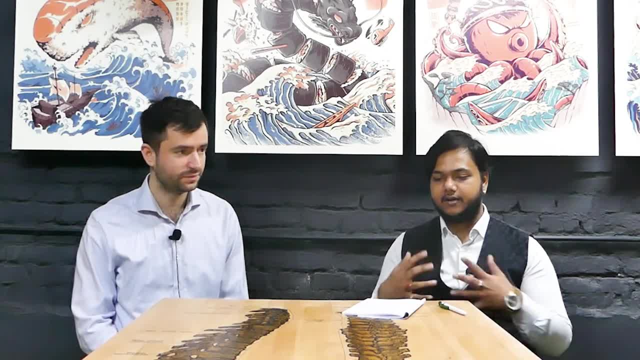 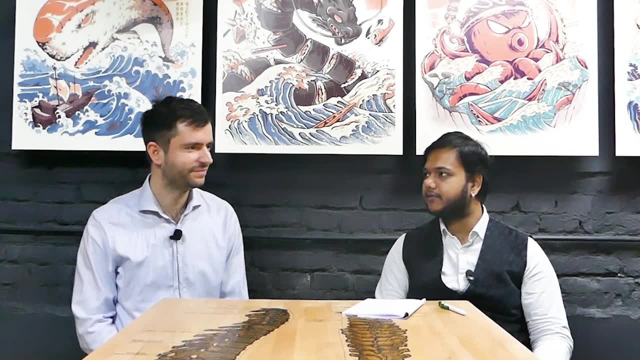 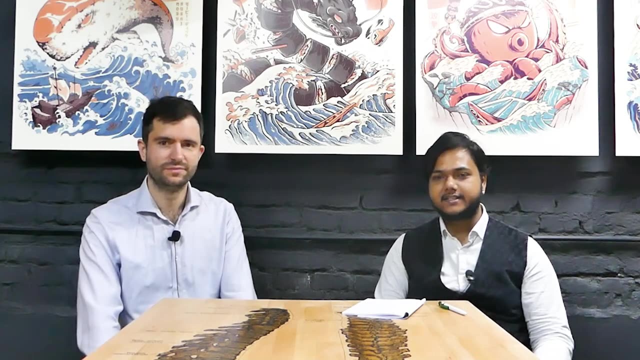 and has good uh relevant connection with the uh companies. uh, we had a discussion a few weeks back with the uh vice dean, mr jan bullets from uh. professor jan bullets from economics faculty, from technical university and he, for example, finds like many relevant opportunities for his international students. he's mostly going. 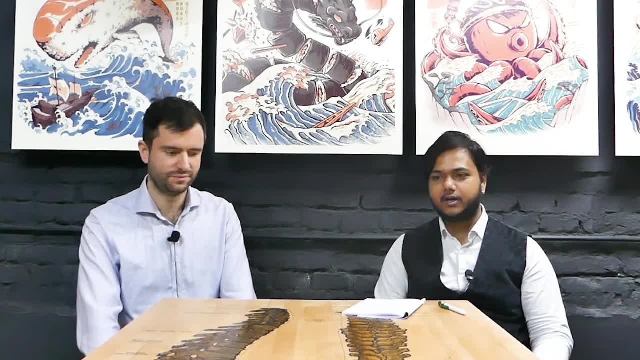 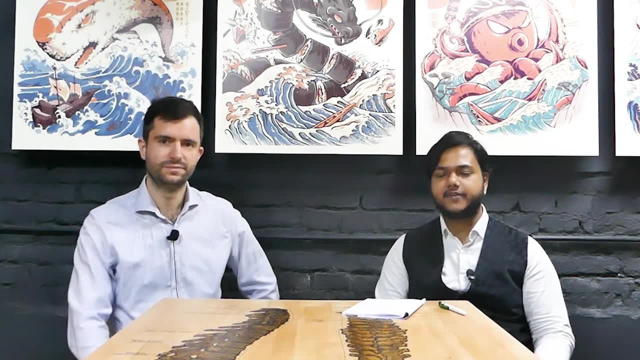 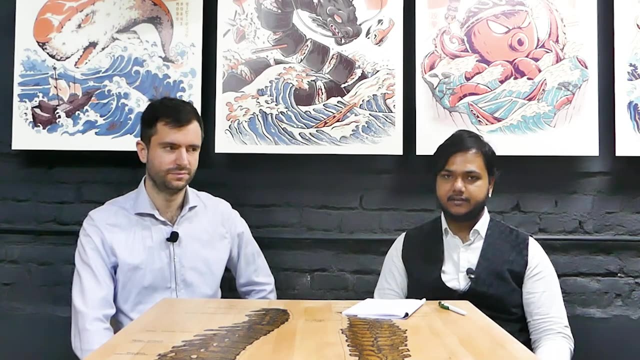 out on this industrial trips and he comes back and mostly offers it to uh the international students, english speakers, so he customized it completely for international students. so generally, like keeping a good touch with your professors, with your dean and everyone who is involved, to you it's a good idea and initially obviously uh. 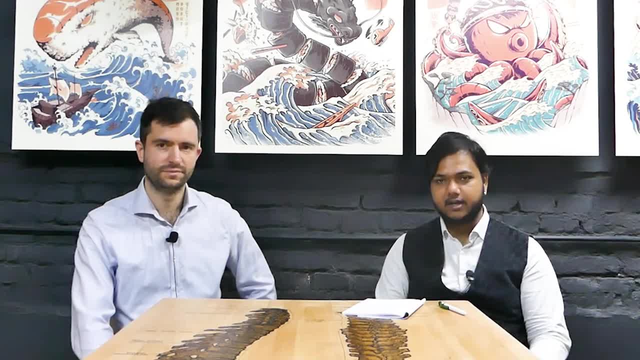 you can start with bolt bolt any of the part-time work. this is going to sustain you for some time. uh then eventually move uh to those. we will link every uh job portal like that are relevant in slovakia in the description, but to mention one of the most prominent one is professia. 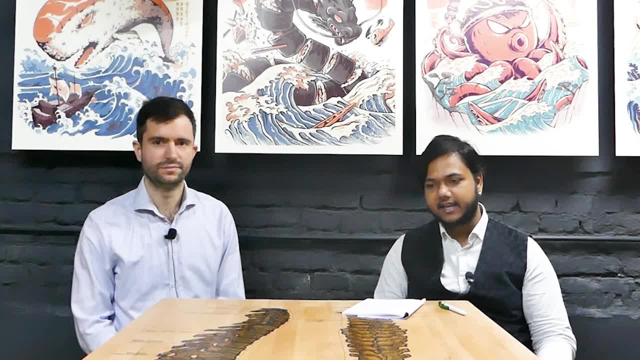 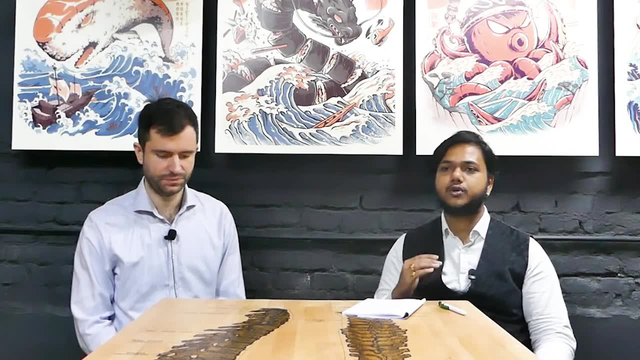 professia has thousands of job uploaded every day, starting from your part-time jobs to nanny jobs to, let's say, ceo level jobs. everything is there in professia. so you should find there are even jobs which are not part-time jobs, which are not part-time jobs, which are not part-time jobs, which are not. 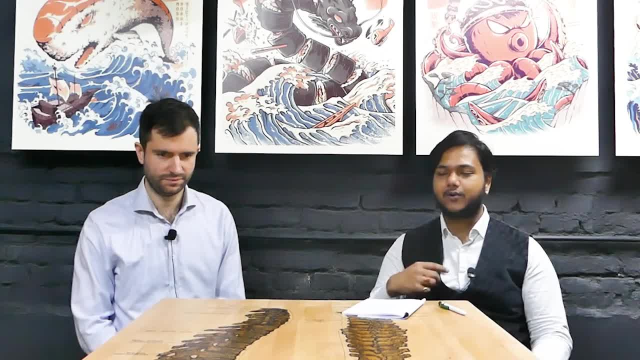 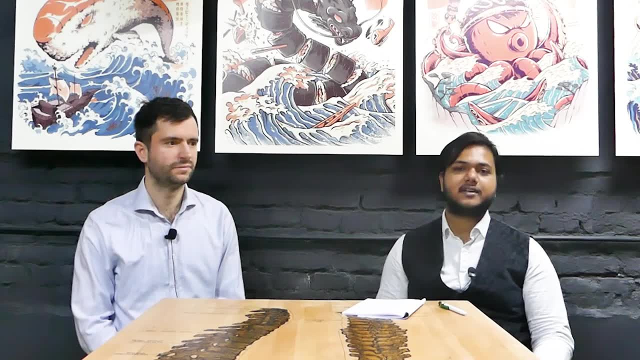 even require you to submit a cv, so you can just straight away go and without a cv, just submit your phone number and write a message and, uh, that goes, and the more you apply. it's a number game. so the more you apply, the more you have chances to find out. there is obviously the general ones, for example: 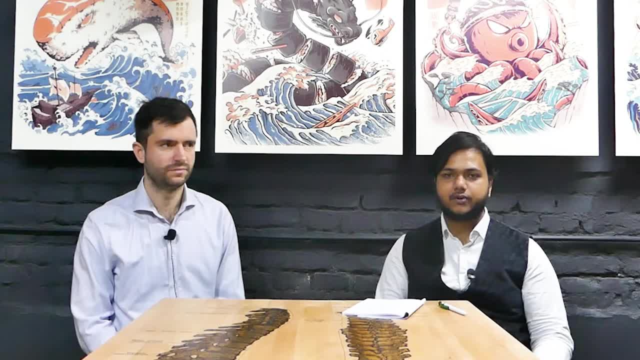 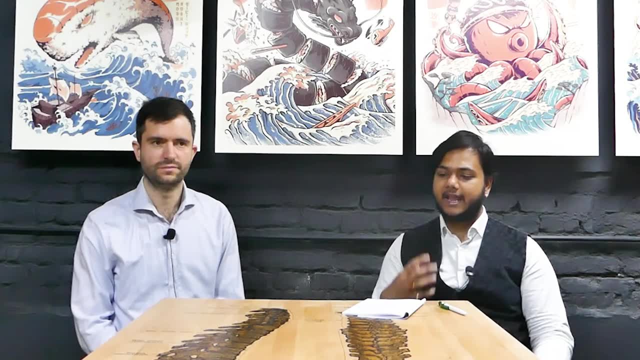 like um the like, linkedin and glassware and all which is more relevant for applying to jobs from other countries or remote work. and obviously like if you're expert in some particular field, like you're a front-end developer, you're a front-end developer, you're a front-end developer, you're a. 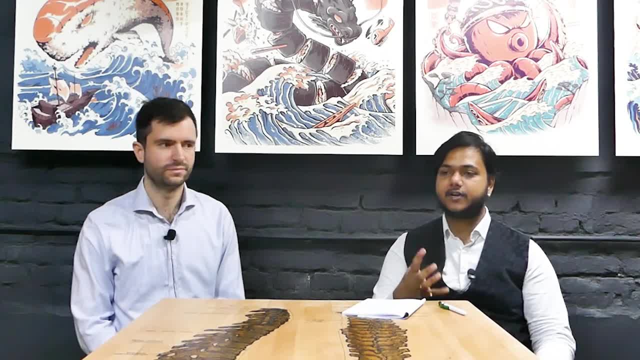 or you're a marketer or something like this. you have some previous experience. you're coming to study masters. in that case, you might also want to open up a freelancer account, something in upwork, fiverr, uh, these sort of websites where you're going to have some freelancing clients and show. 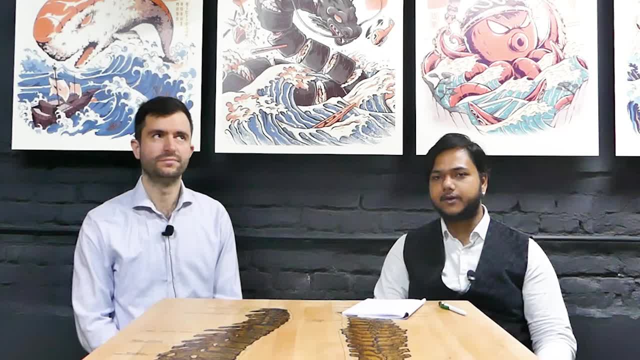 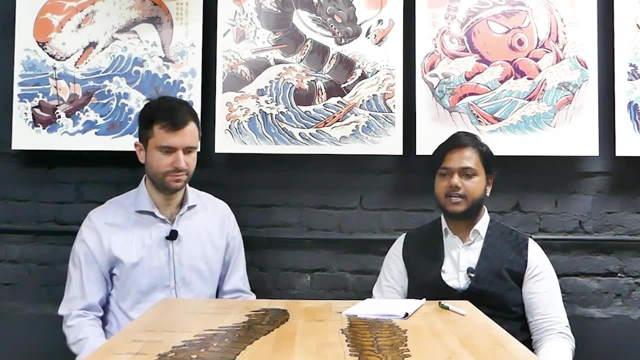 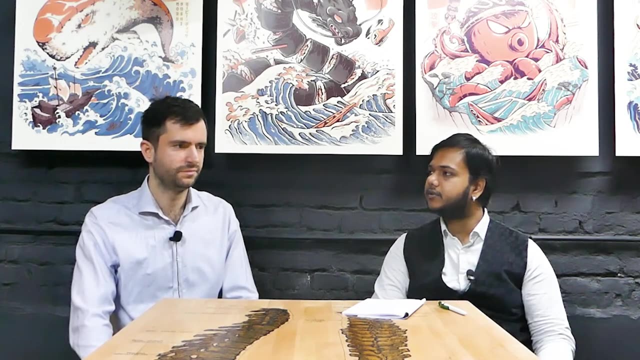 even like the slow clients that uh, you know you're doing some relevant work and get some clients from there. so these are the different income sources, but in general what we would say uh on an average, like uh compared to the living expenses in slovakia, how much would you say a student, uh, living normally, you know, like a standard life would. 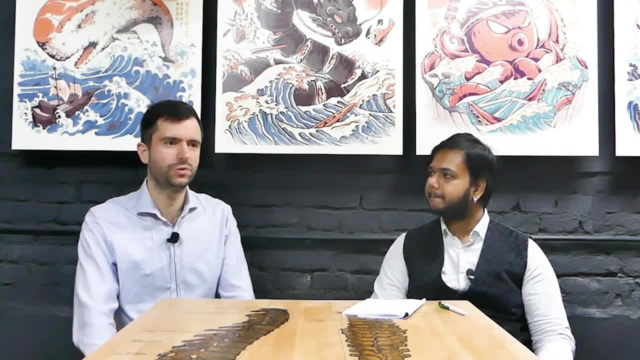 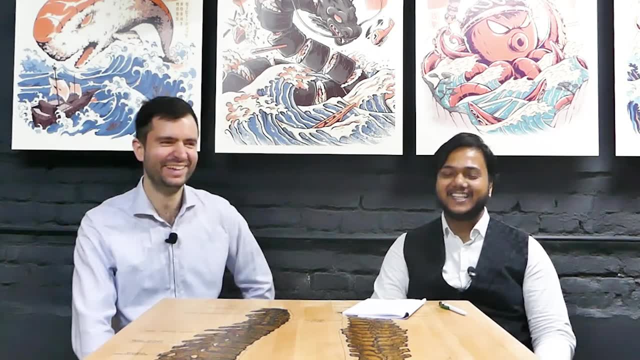 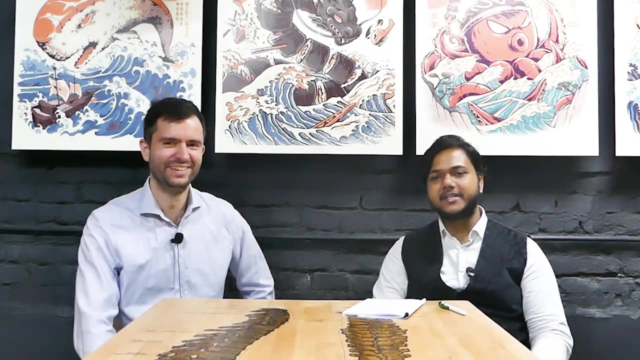 spend living in a dormitory. living in dormitory, i would say 300, if he doesn't smoke and drink too much. okay, that's a, that's a very important disclaimer: do not smoke and drink too much. but okay, like three to five hundred is something you can expect, like, uh, in a month to spend. 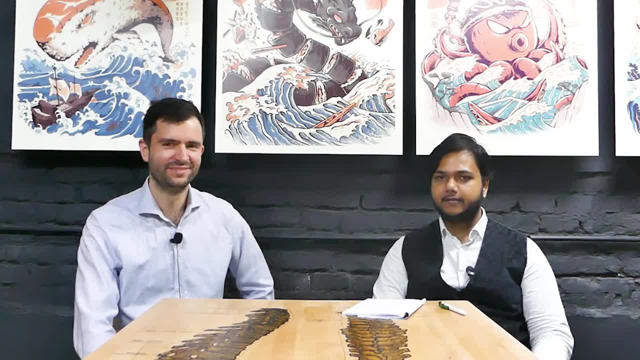 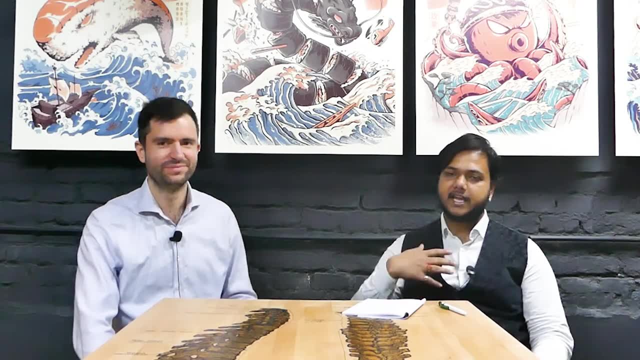 and this income. for sure, with any of the part-time jobs you should be uh able to find out, um able to generate uh. but yeah, uh, there are more scopes, there is more opportunity and eventually, when you move to full-time ones, you can make much more uh money than this. so, uh, anything else you would. 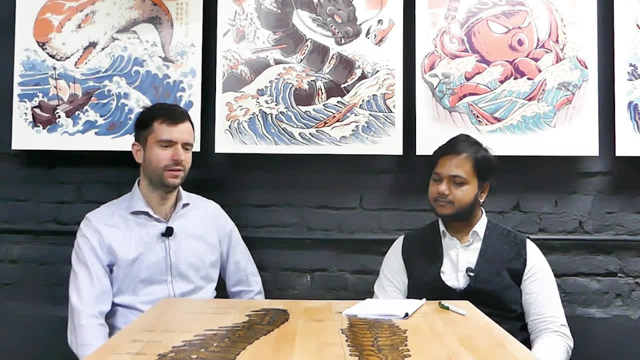 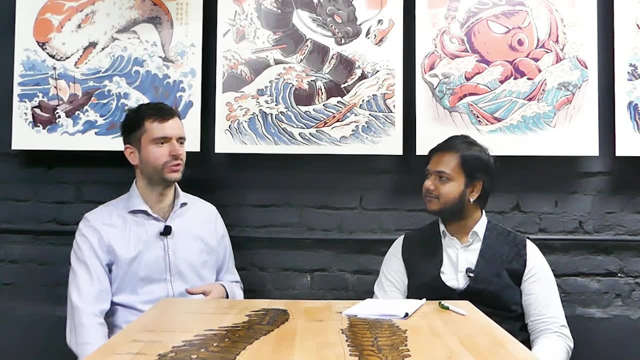 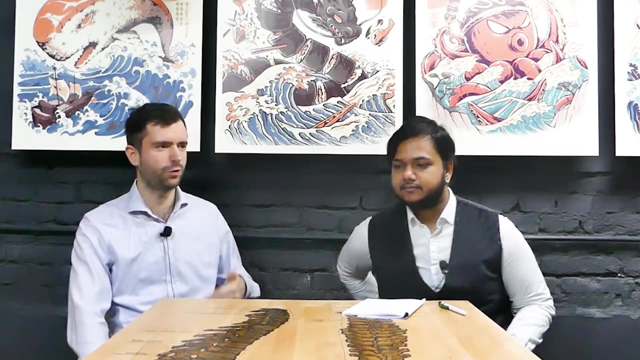 like to add for our viewers. yeah, so i would say, um, i would like to make also one note because, like things, they keep changing in time. so, yes, it currently, as you saw, like the getting like residence, uh permit for job, it's quite difficult uh doing things properly uh. 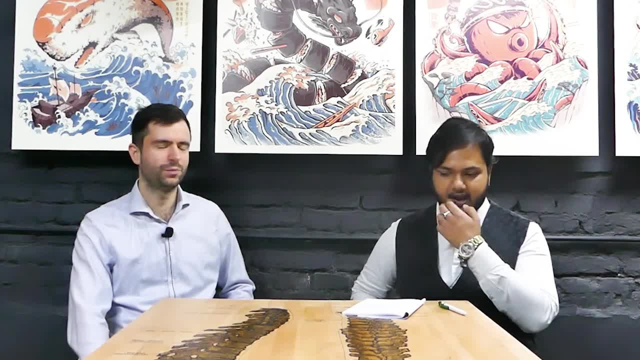 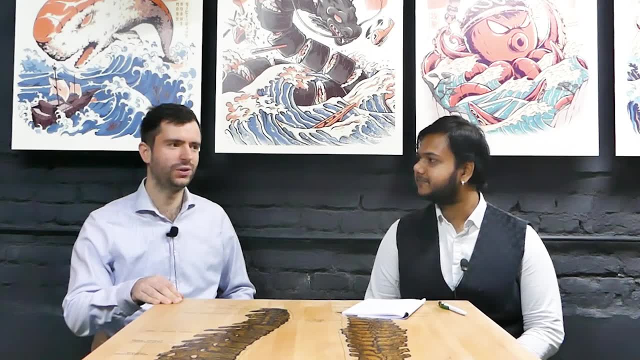 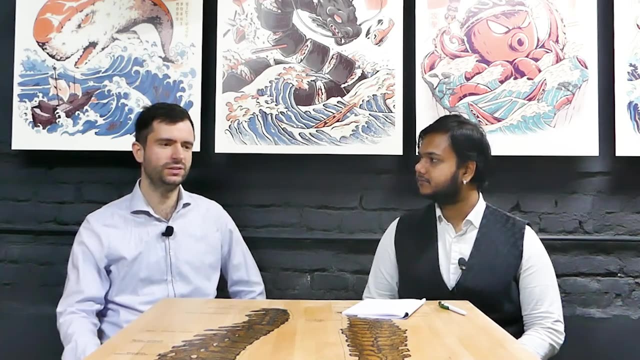 work here. it's quite difficult, but um, like the current prospects, um, uh, like slovakia, it's aging country, uh, and there are, like many companies, mechanical companies, automobile companies, uh, remote centers and so on. so these companies, they will be forced to hire someone if they don't. 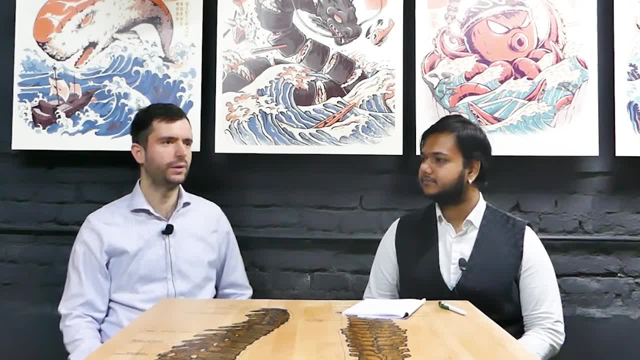 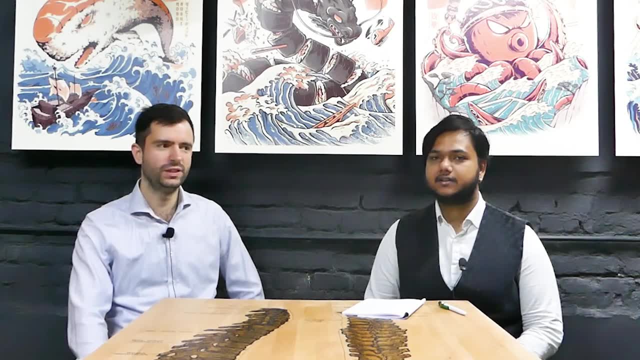 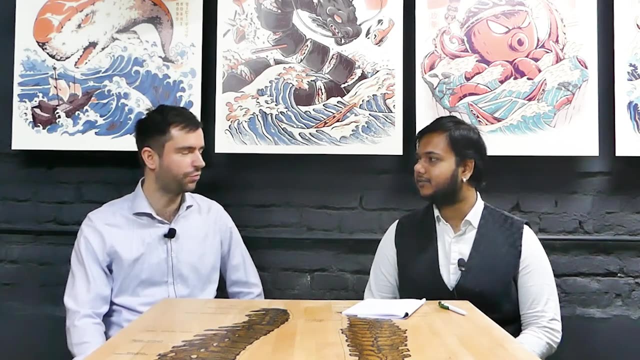 want to close themselves. yeah, so it's expected that approximately 100 000 people will retire by to 2030. oh wow, six years. so these companies basically will have either chance to adapt or to stop working. so i'm pretty sure that also the rules for incoming workers, both qualified, 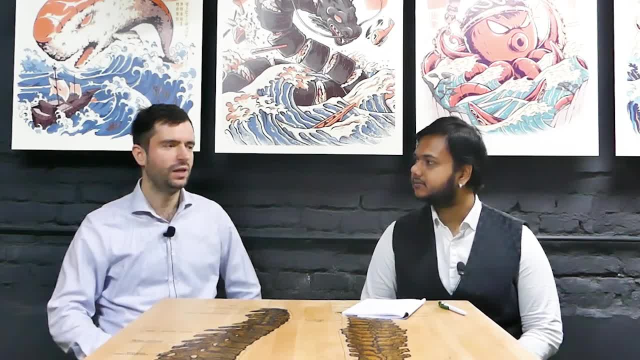 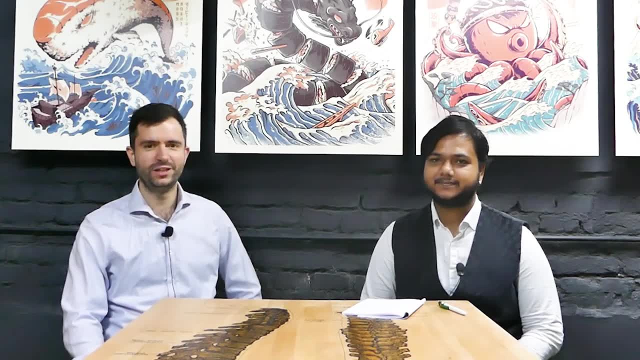 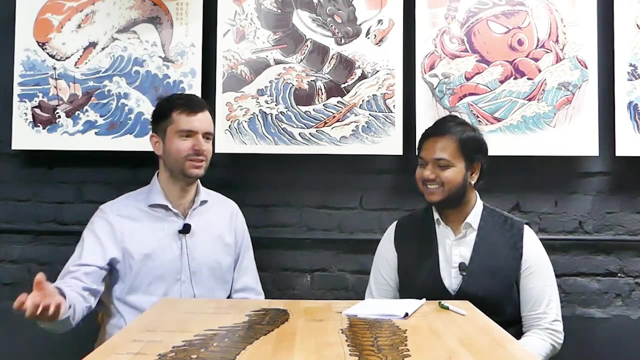 non-qualified will change rapidly, yeah, next years, because basically, if you have like retired people like you need to pay their health pensions and so on, and for that you need, uh like workers and, of course, taxpayers, taxpayers and of course, like i can imagine, these people will be still interested to come to slovakia to work. 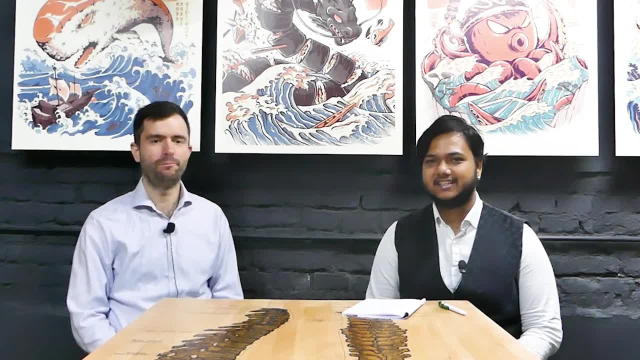 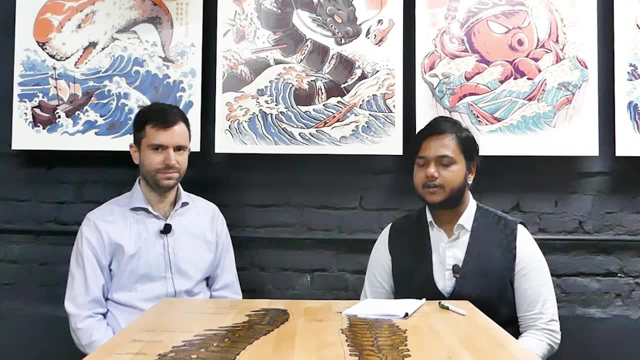 so it's just matter of few months to years until the immigration rules will change rapidly, absolutely, uh. but i would like to mention one thing over here, uh, which might be relevant. that is, uh, generally: if you're coming uh in europe already to study, to find a job, settle in for a. 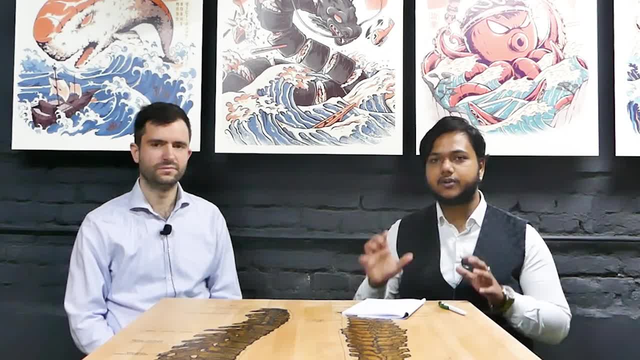 job is much easier than if you have a phone number that is relevant to the phone id code in slovakia or in europe, and then you can go to slovakia and you can go to slovakia and you can go to any of the european countries. it means you are already residing here. your visa processing should. 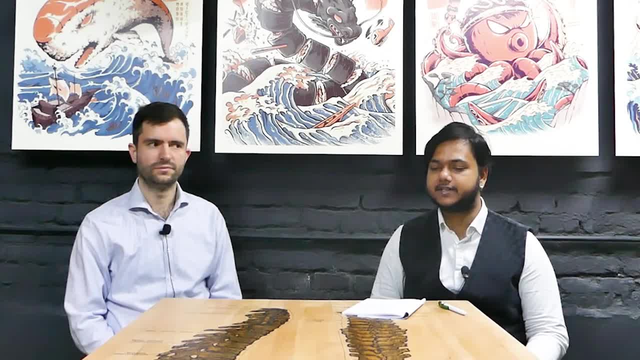 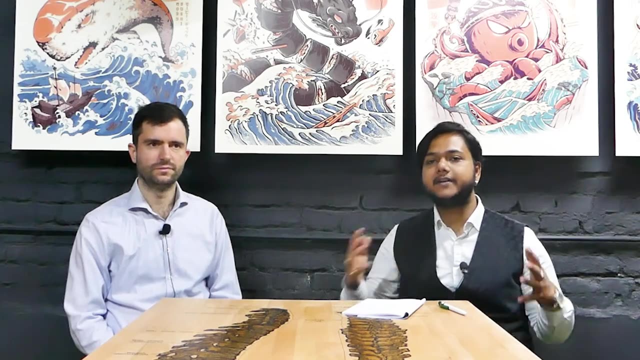 be much easier. visa residence card processing should be much easier in that case. what they do is like they instantly respond to you. they go through the normal application process, normal recruitment process and everything, whereas if you're applying from india or you're applying from china or any other country, it's a complete visa process. it means you have to go and submit. 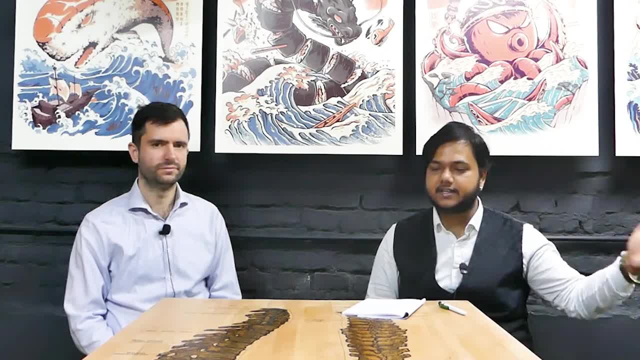 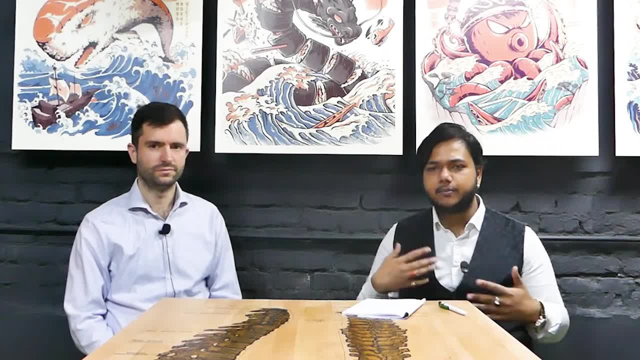 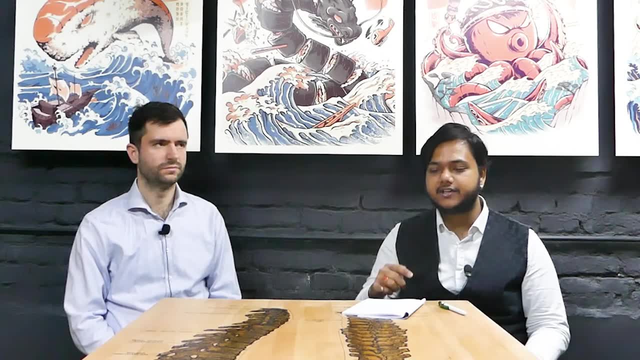 it means in general, it's a like you know it goes as a rejection. you might even have seen it. when you apply on linkedin, on any or any website, they ask you that, are you eligible to work in this country? you put yes, you need a sponsorship of this country. when you put yes, it's generally the. 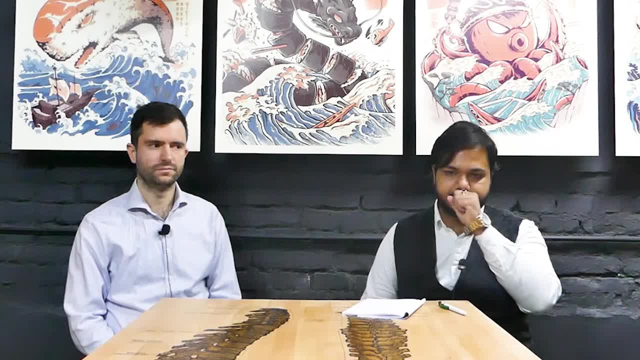 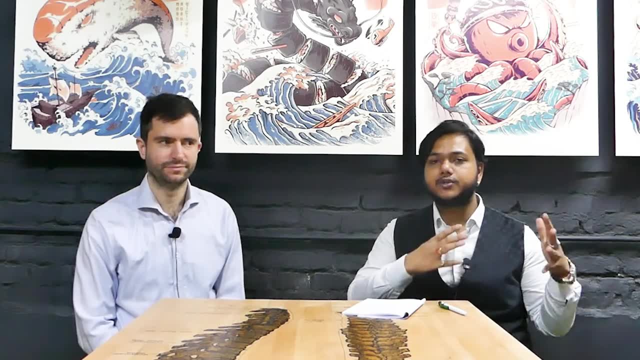 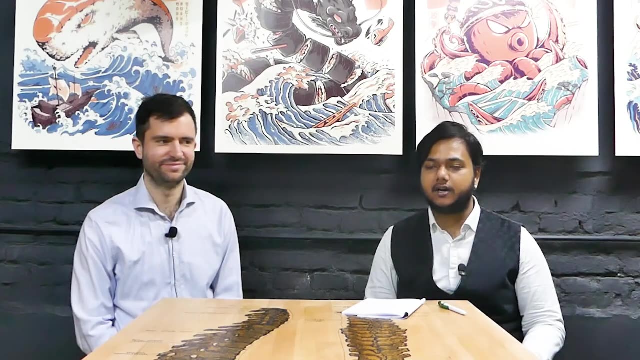 ats itself like throws a rejection on you. so that's why, if you're planning to study, or if you're working now in some other country, plan your study in europe so you can have a smooth transition to some jobs. your network is much better if you actually like work here and study here as well. so then you have. 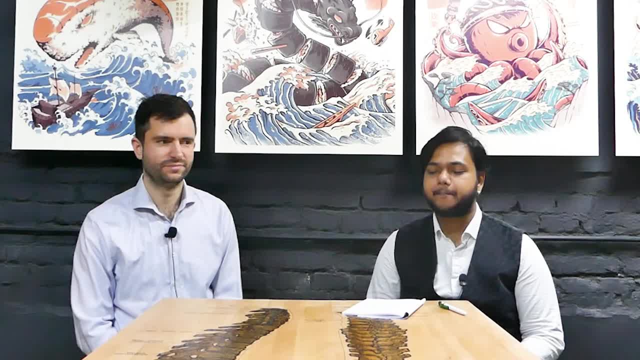 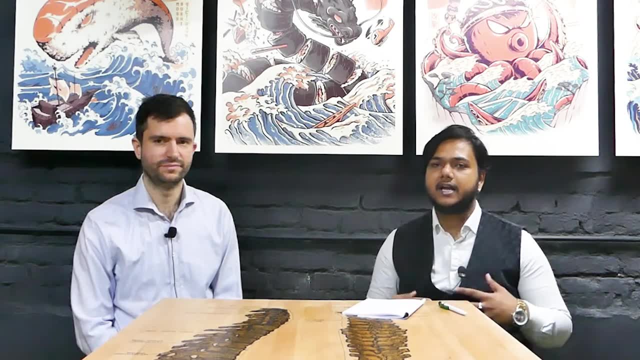 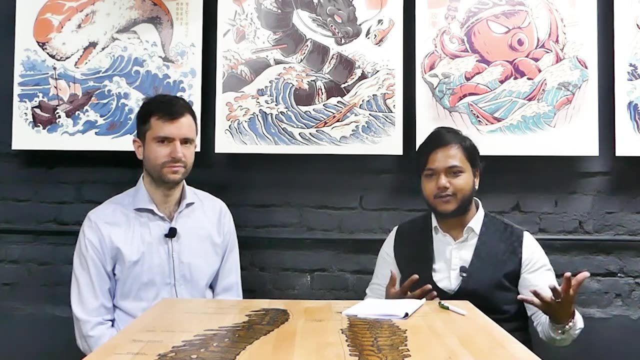 more opportunities, much more things popping out at the same time and yeah, and also these connections are going to help you. but the most important thing is also that these visas that you mentioned about in general european countries have this and you will see plenty of reels and plenty of- you know like um- videos about this. like luxembourg wants people germany wants. 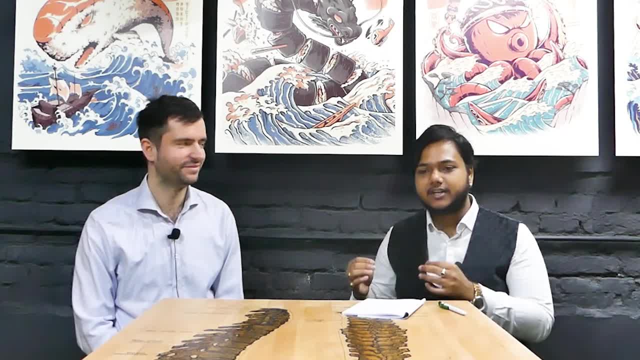 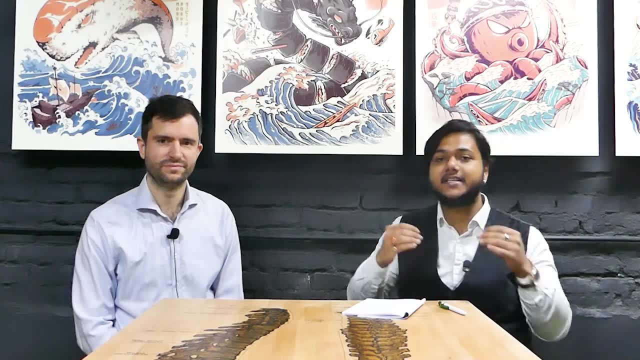 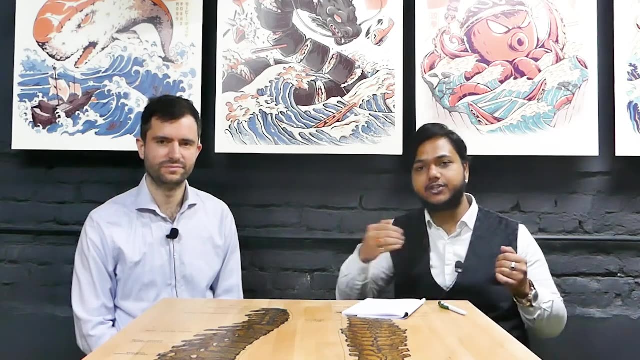 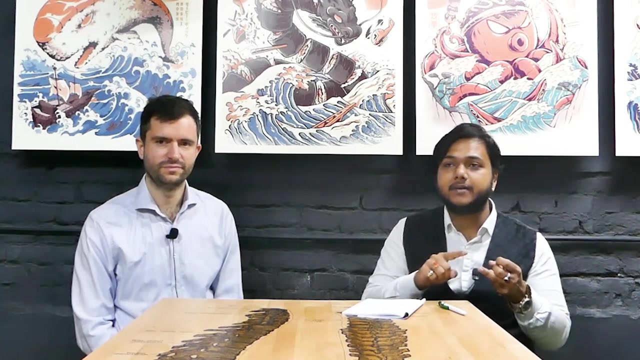 people and, trust me, these are actually like some agency advertisement and these advertisements are for specific fields with people with specific expertise and experience. this is not in general, so the general thing is it means, if you work in any general field, not in these specific fields. these specific fields can consist of, for example, pharmacy. can consist might be of cyber security. 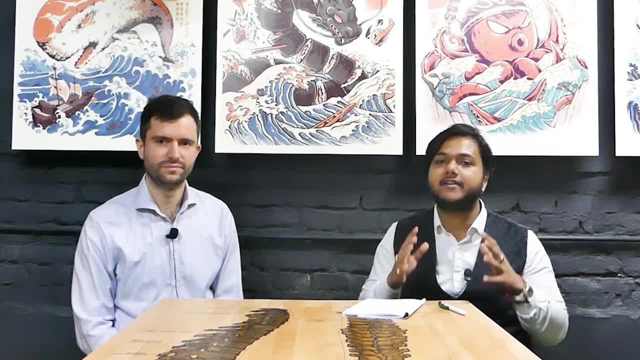 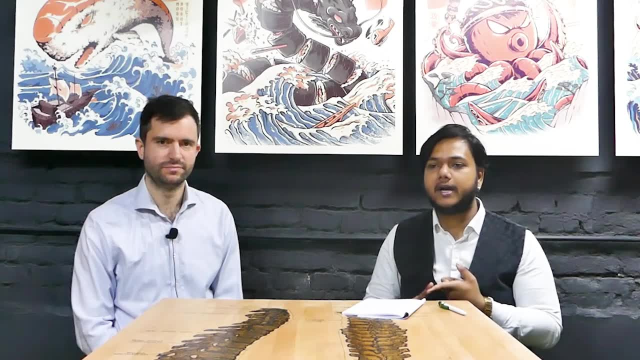 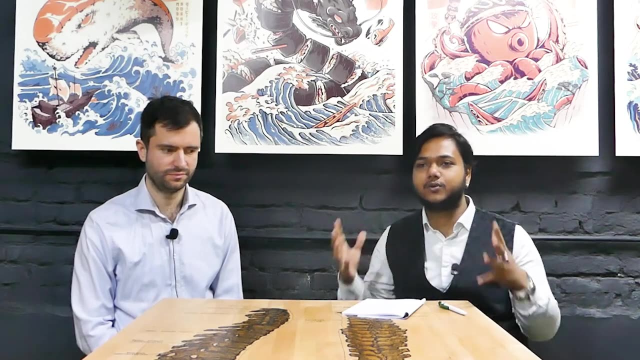 can consist like, and it has also experience level requirement. it means you are working as a cyber security developer for minimum five years, you are working as a, let's say, automobile production engineer for minimum three years. it might have something like this, and those people are required, let's say, in two thousand, four thousand or six thousand. it 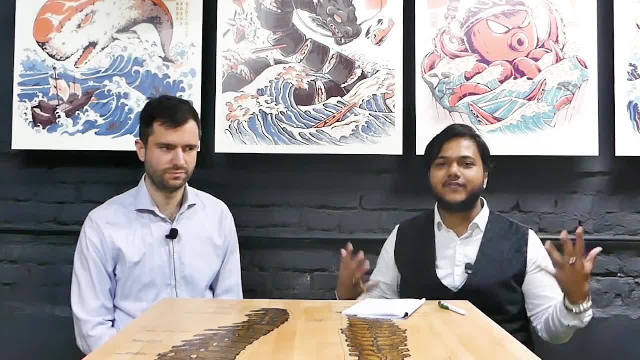 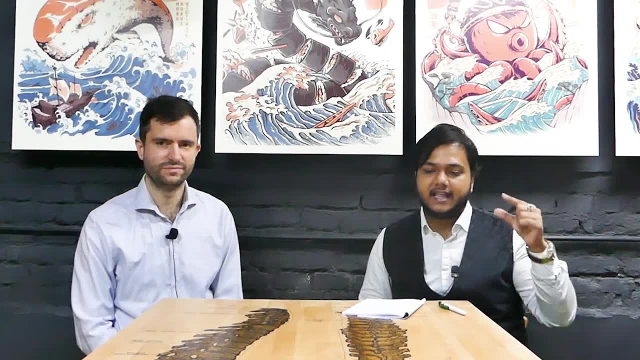 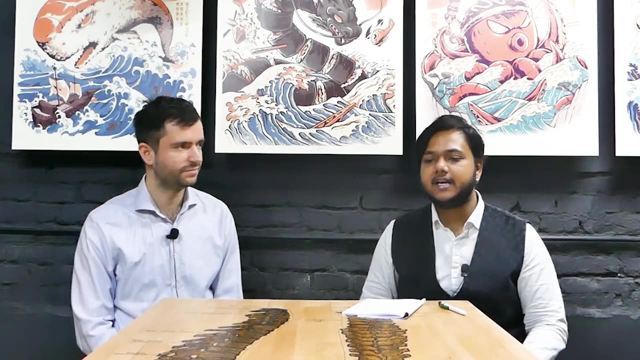 doesn't mean that luxembourg or slovakia or germany all of a sudden requires like fifty thousand people with plenty of job. it's not. it is like only relevant to these particular fields, and these are generally- they're uh portrayed or mentioned in the uh websites or the labor ministry's website: the high, uh highly skilled migrant or uh this highly 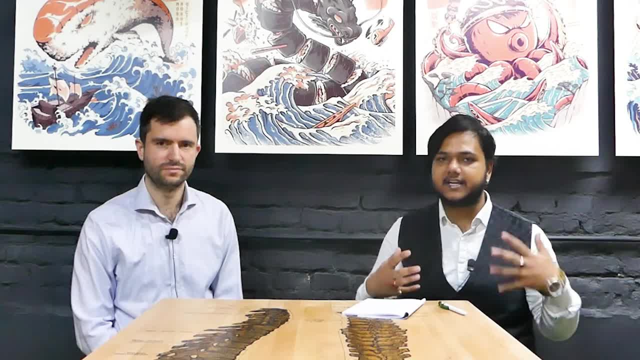 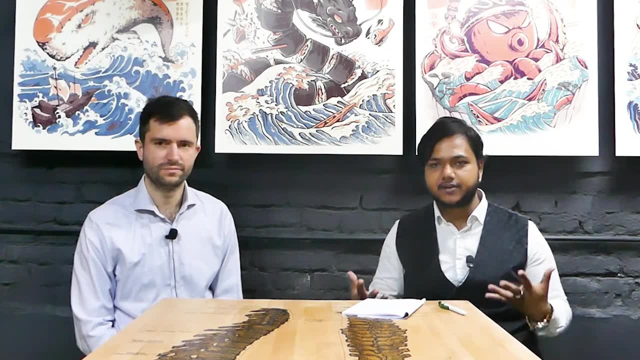 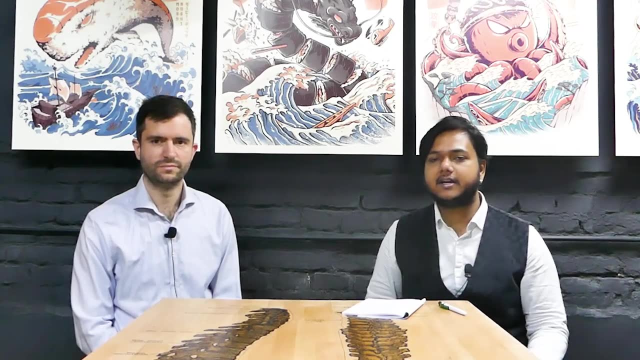 demanded uh fields, but the rest are still competitive. it means if you're working in sales, marketing, accounting, economics, finance, any of these sort of like general fields, or even some of the engineering fields as well, and this is like, so you have to go through this process until and unless in that particular field there is like high demand of labor. yeah, it means that. 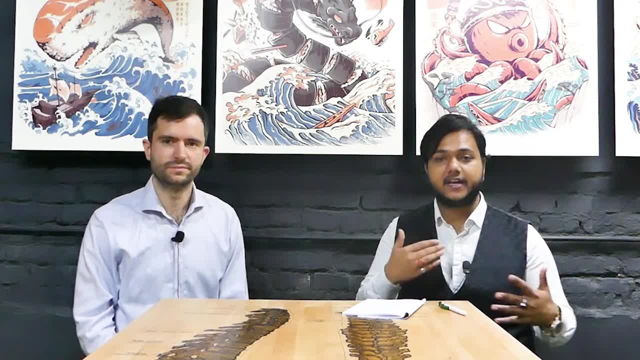 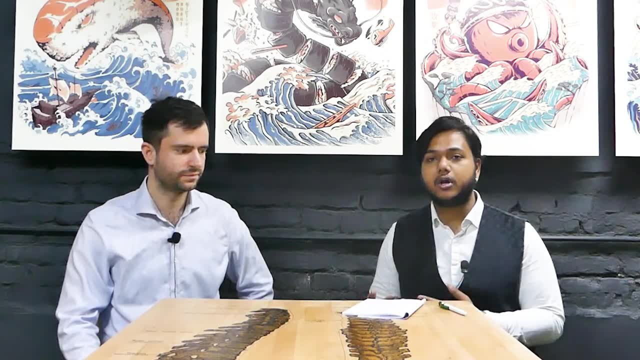 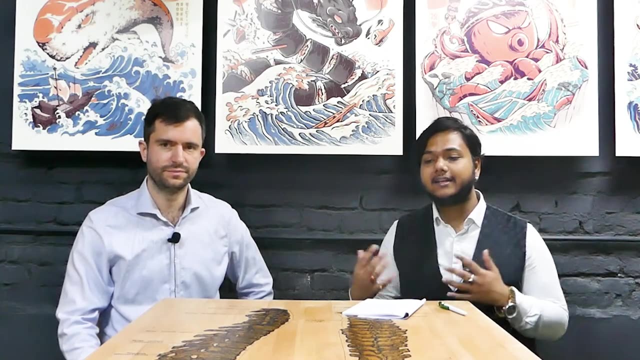 these jobs are available, uh, but at the same time it is very competitive. but the easiest way is if you already move in euro. in general, people who are hired from abroad are two cases: one that already are here because of studies or something like family or something like this, or the other cases they have really so much experience or expertise. 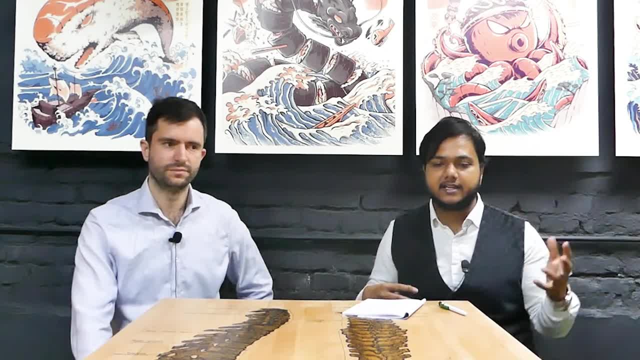 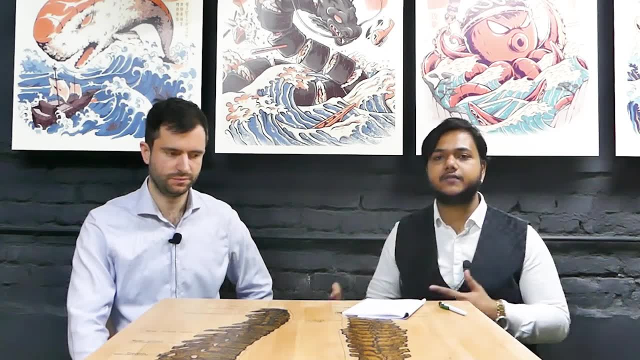 like 10 years plus or five years plus with like specific field, like, let's say, blockchain or something like this. that is the only case that they are hired and all the company is willing to wait for you to. you know, come to euro and start working. other than that, if you're working in a general, uh field, let's say like: